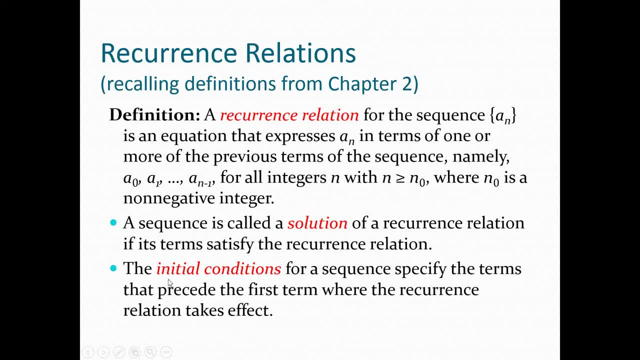 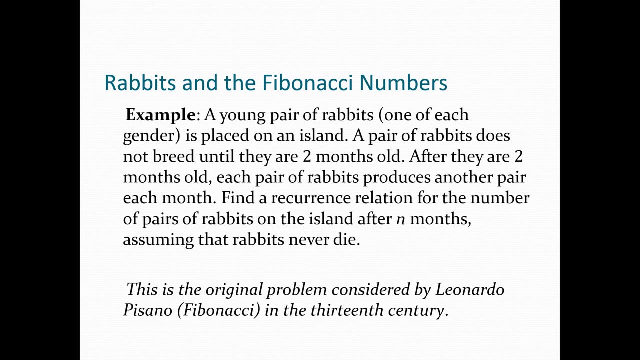 and which satisfies the recurrence relation, And the initial conditions for the sequence specify the terms that precede the first term where the recurrence relation takes effect. So, first example, how to build a recurrence relation: A young pair of rabbits is placed and these rabbits, one of 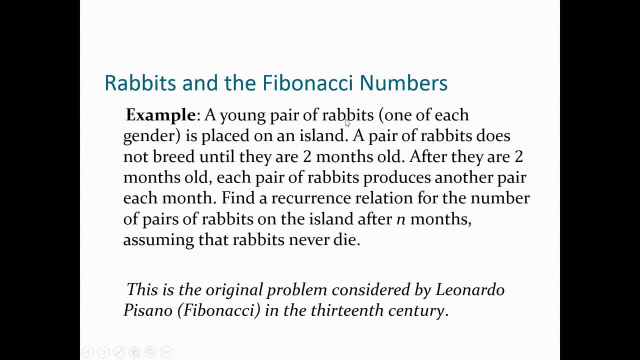 and which satisfies this brilliancy gender? okay, this is important to note- that is placed on an island and a pair of rabbits does not breed until they are two months old. After they are two months old, each pair of rabbits produces another pair each month. Find a recurrence relation for the number of pairs of rabbits. 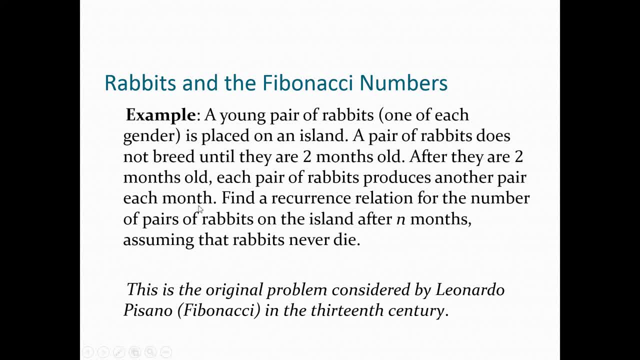 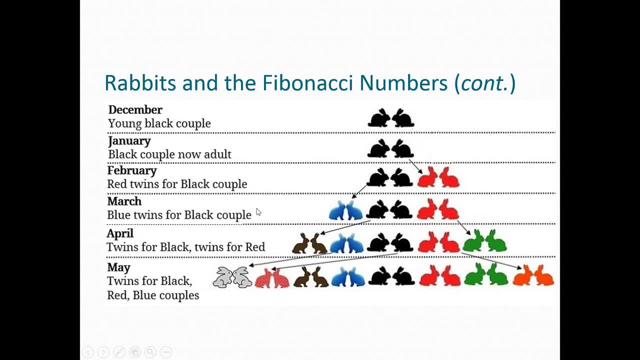 on the island after n months, assuming that rabbits never die. So this is an ideal situation that rabbits never die. So let's see. how does it work? So if we have, if we start from the first month, let's say that first month be in December. So we have one pair of 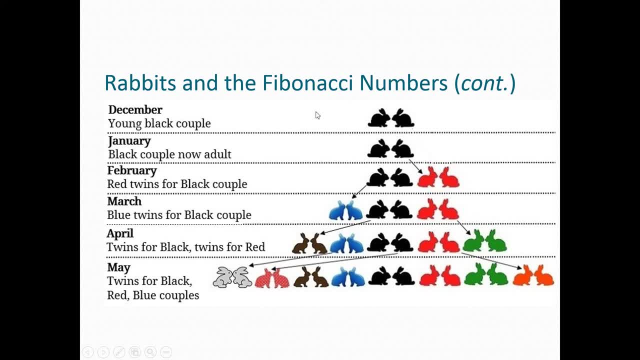 rabbits, which is a young pair, okay, So after first month it's not able to breed. So then we still have one pair of rabbits. So now this: after two months it becomes adult and now it can breed. So in third month we have two pairs of rabbits. one, the old, 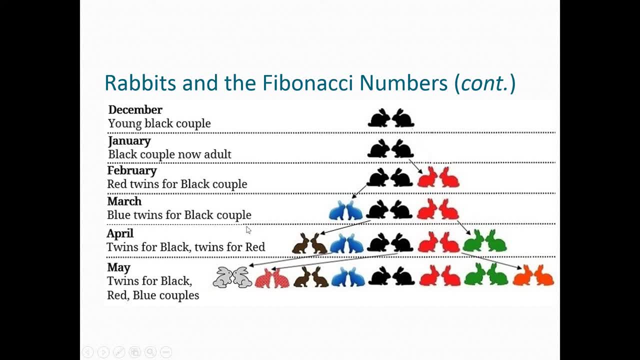 pair and one the new pair. ok, So in the fourth month now this new pair is one month old, so it cannot breed, but it cannot breed every month, but this old pair can breed every year, months. so one pair, the pair itself and a new pair comes again in March. so we have 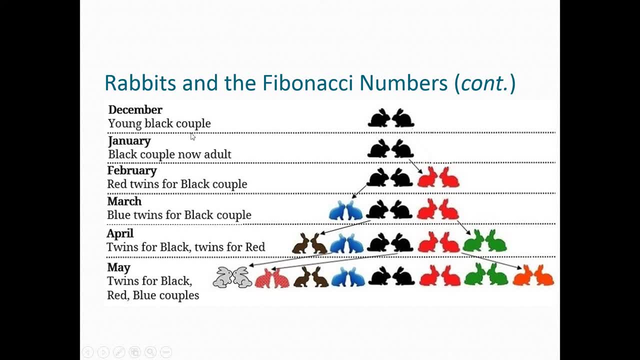 three pairs are in fourth month, okay, so in fifth month. so this is an adult pair already and this pair is also two months old now and it can breed. so there is a new pair from this red pair as well and from a black, from old black pair we have. 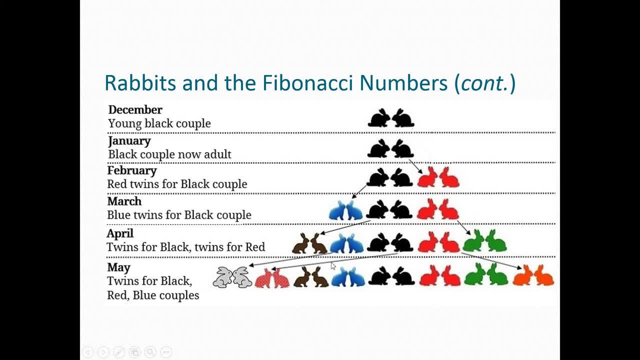 a new pair again. so, and and this blue pair is one month old, so it cannot breed, so it remains one pair. so now we can we have one, two, three, four, five pairs. okay, and similarly, in the sixth month, that is, in May, we have one, two, three, four, five, six, seven, eight pairs. now, if you see the 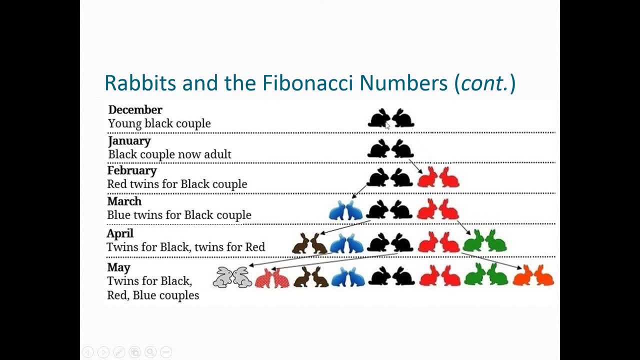 pattern: in first month we have one pair. in second month we have again one pair, but in third month we have two pairs. okay, one plus one is two, right? so we added the pairs, the number of pairs in previous two months and we have the number of pairs in third month. okay, 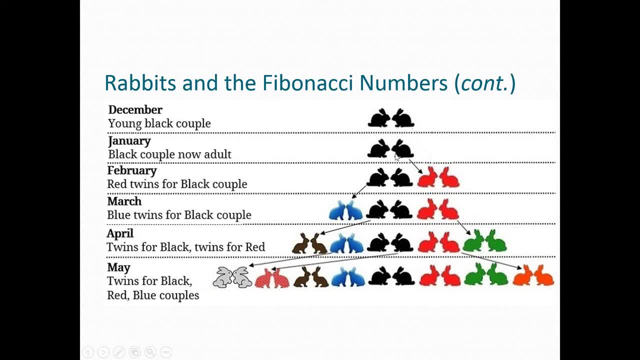 now in fourth month, again the see the pattern. in the third month we had two pairs, and the second month we had one pair, and now add both of them, we have in total three pairs. so in next month we have three pairs. okay now, in the previous month they were two pairs, so add them. we have a total of three pairs equal one of. 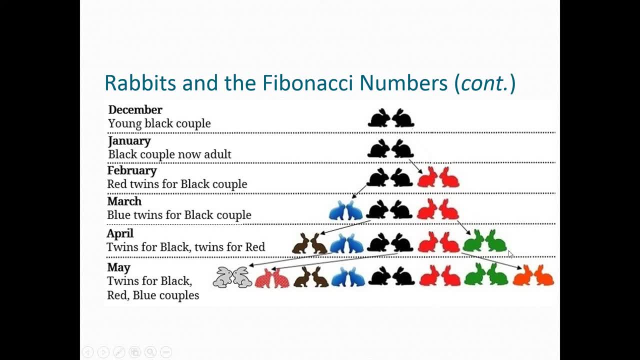 five pairs. so in next month we have five pairs. so this is, this is the pattern. similarly, when you add these total number of pairs in these two months, so we have the number of pairs in the next month. so one, two, three, four, five, six, seven, eight. okay, so five plus three is eight. now in the sixth month we have one. 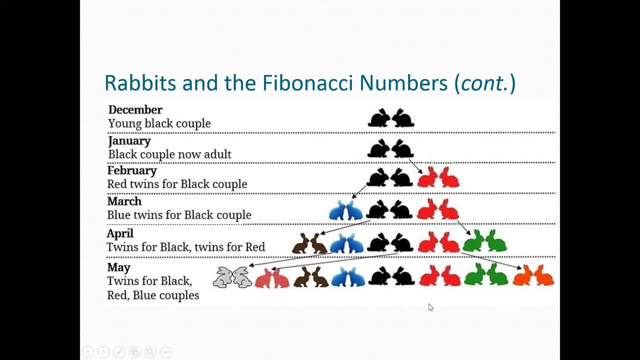 two, three, four, five, six, seven, eight. so it means in the nth month the total number of pairs is the sum of the number of pairs in n minus first and the number of pairs in n minus second month. right, so here we go. so detail is given in. 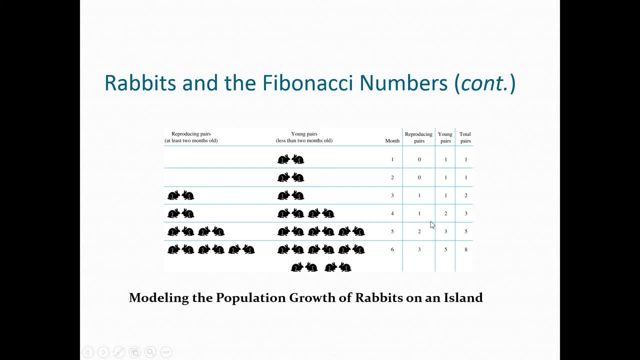 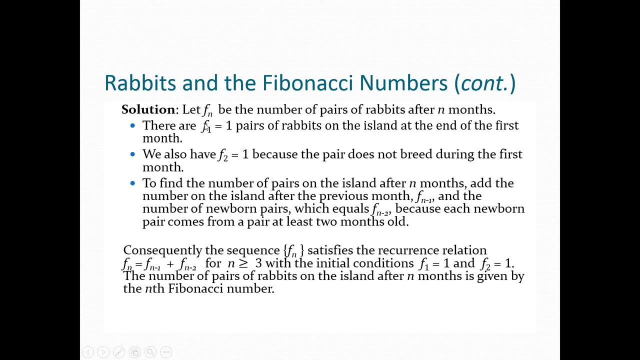 numbers here you can see, and this picture is taken from your book so you can see it. whatever I elaborated in the previous slide, it is written here. okay, so the solution of the problem. so this was actually the pictorial view of the problem, and now the solution, mathematical solution. let fn be the 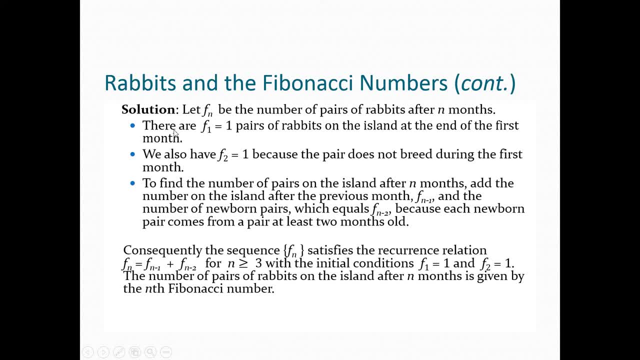 number of pairs of rabbits after n months. so they are f1. that is number of pairs in first one-month f? n with the number of pairs of rabbits after n month. so f1 represents the number of pairs after one month, which is one. okay, one pair of. 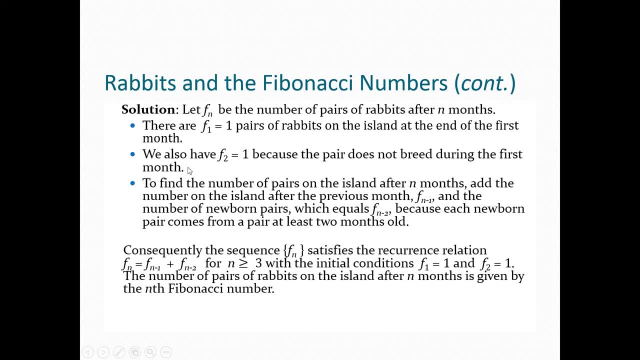 rabbits on the island at the end of the first month. so again, we just discovered that at the end of two months we still had one pair, because the pair does not breed during the first month. so to find the number of pairs on the island now to end months, mm. 2, ie, what is? ie the guessing marks. 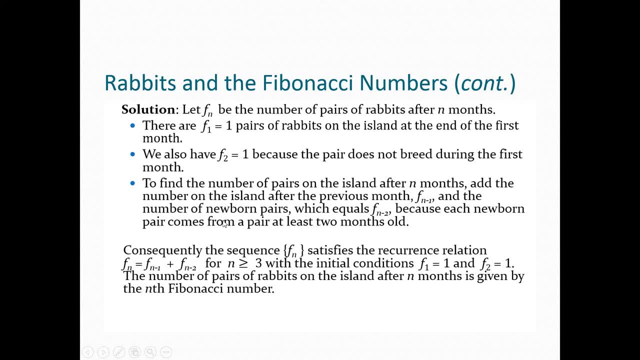 on the island after the previous month, fn minus 1, and the number of newborn pairs, which equal fn minus 2, because each newborn pair comes from a pair at least two months old. So consequently, the sequence fn satisfies the recurrence relation. fn is equal to fn minus 1 plus fn minus 2.. 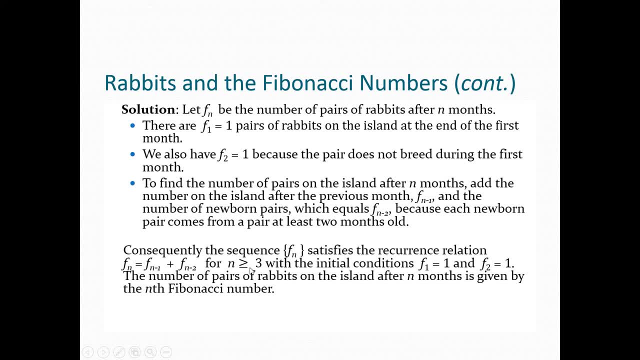 Now for the condition on n: n is greater or equal to 3, because this subscript must be non-negative. okay, So if we know the initial two values, so in order to find third value, we have to put n is equal to 3.. So n is greater or equal to 3.. So when n is greater or equal to, 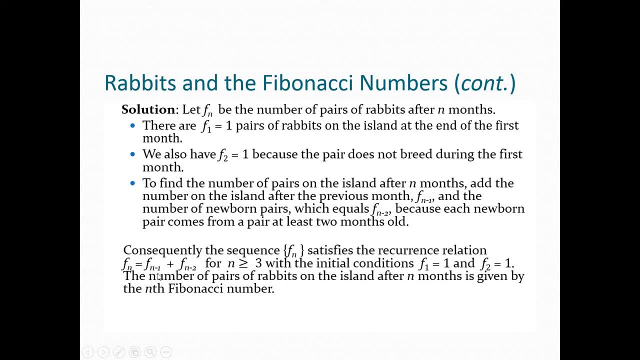 3 we have f3 is equal to f sub 3 minus 1, f sub 3 minus 2.. So, which is f2 plus f1, which is 2, okay, So f 3 is equal to 2, and so on. So this is the solution of the problem. The number of pairs: 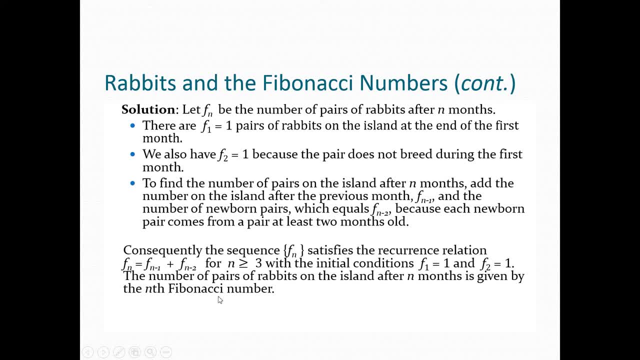 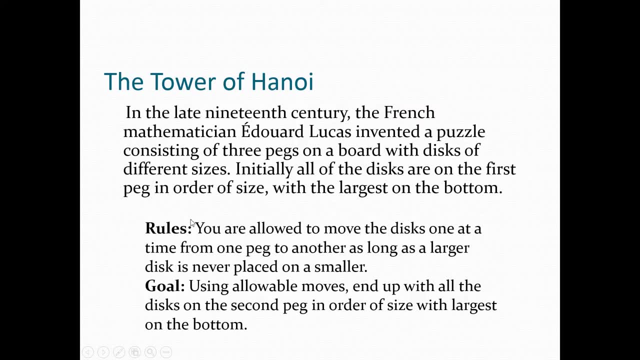 of rabbits on the island after n months is given by the nth Fibonacci number. So these numbers are called Fibonacci numbers. Now there is another problem: the Tower of Hanoi. This is a very interesting problem. In the late 19th century, the French mathematician 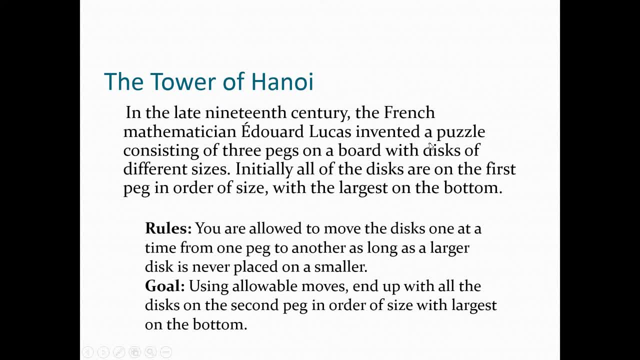 Edouard Locus invented a puzzle consisting of three bags on a board with disks of different sizes. Initially, all of the disks are on the first bag in order of size, Now with the largest on the bottom. So rules are rules to rearrange the size of the disks. 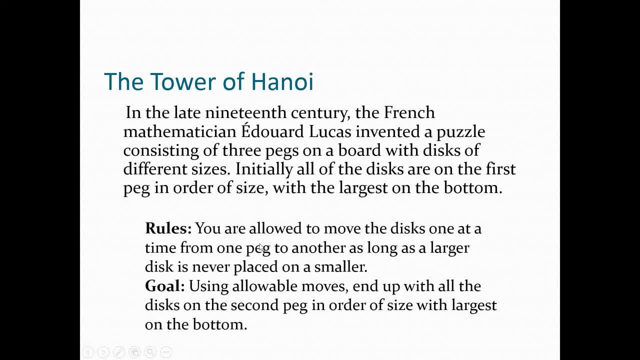 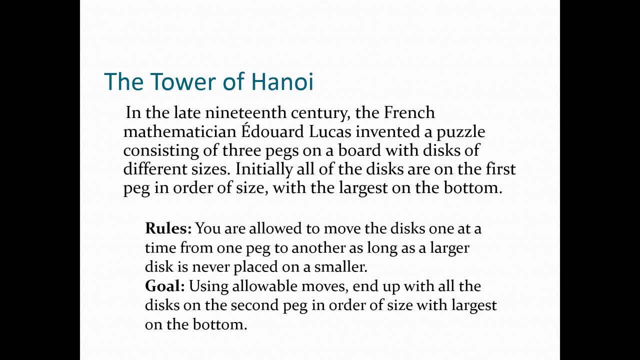 disks, one at a time, From one bag to another, As Long as the larger desks are never placed on the smaller. So this is the rule that the larger kau integrated disk is never placed on a smaller. Okay, goal in this problem is using allowable moves. end up with all disks. 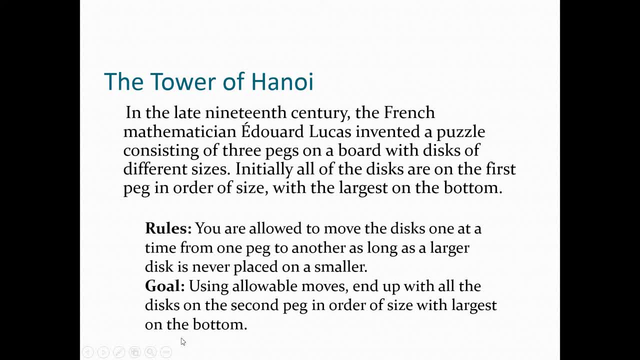 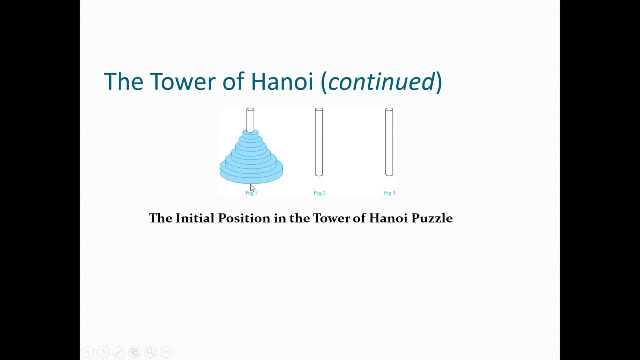 on the second bag in order of size, with largest on the bottom. so let's see, initially we have all the discs placed on the first bag, like this, and we have to move into, move to one of the these two bags: bag two, you may say, or bag three. 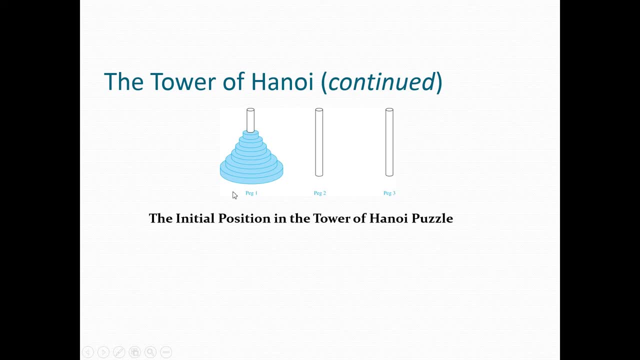 one, one of the bags, and we should keep these rules in mind in order to achieve the goal. so let me show you few animations- how does it work? and then we'll generalize. so here we have. so if we have two discs, how many steps are required to shift these two into this bag? see so 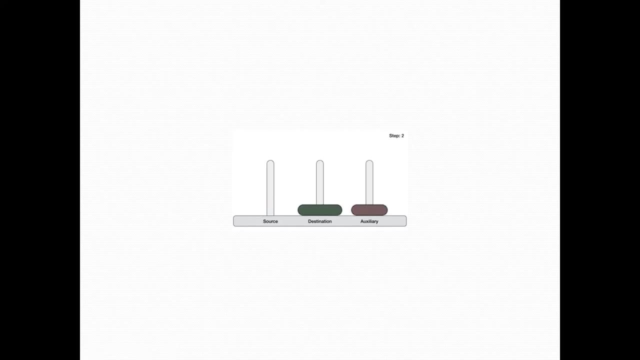 let's count one, two and three, we're done. okay, so, in order to shift, we have, only three steps were required. okay? so let's see: if we have three discs- one, two, three, four, five, six, seven- so seven steps are required, and if we have four discs, then 15 steps are required. keeping all the 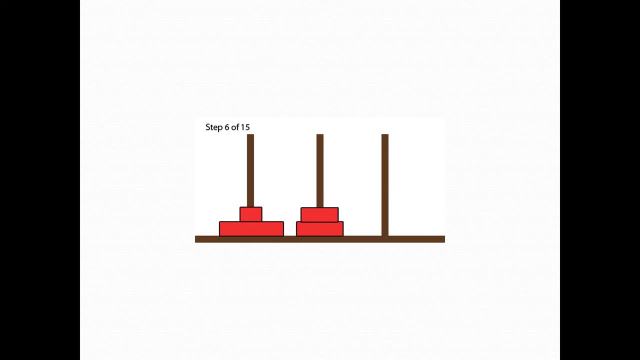 rules in mind. okay, see, yes, yes, yes, yes. third one is yes, yes. 2nd 1st: Yes, this is step 8, and then step 9, then step 1011, because larger risk cannot come over a smaller risk. so in step 15 we are able to shift all the discs to. 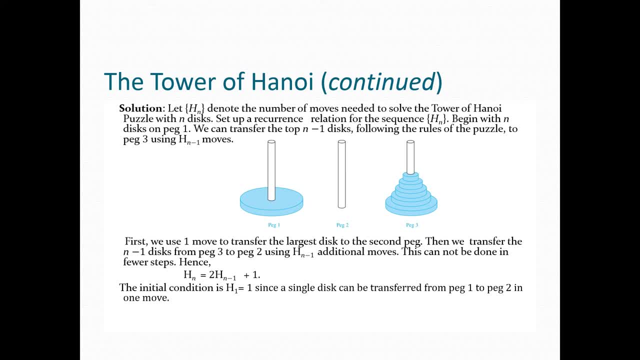 the other part. okay, budget this. bags the other pack, however big for the mathematics, into find you the? so, uh, let h? n denote the number of moves needed to solve the tower of hanoi. okay, so we have n disks, and let h? n be the number of moves needed to solve the tower of hanoi puzzle with n disks, okay, 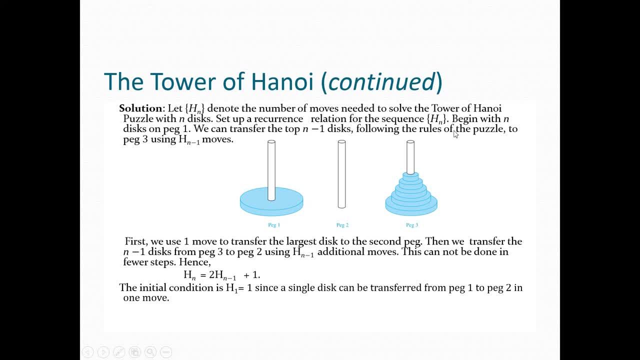 so set up a reconciliation for the sequence h n begin with n disk on begin with n disks on peg 1. so, uh, like this, we have n disks on peg 1, okay, so we can transfer the top n minus 1 disks following the rules of the puzzle, to peg 3, okay, using h n minus 1 moves. so h n moves are required. 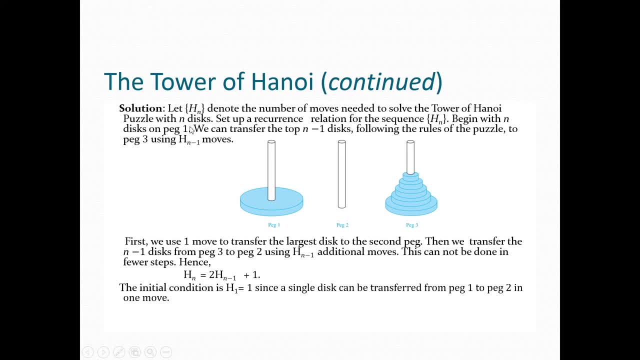 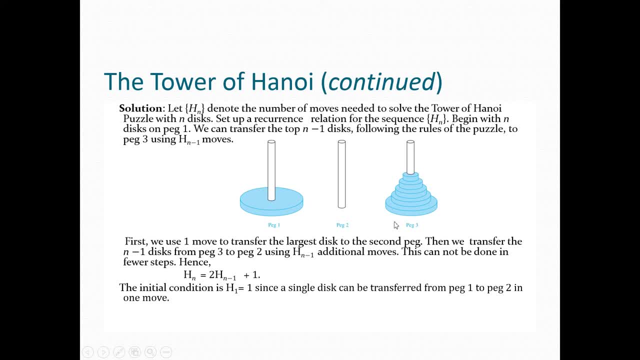 and the smallest one is on top. So how many ways are there to rearrange these disks? is h, n minus 1? because n minus 1 disks are arranged, So h, n minus 1 moves are required to arrange n minus 1. 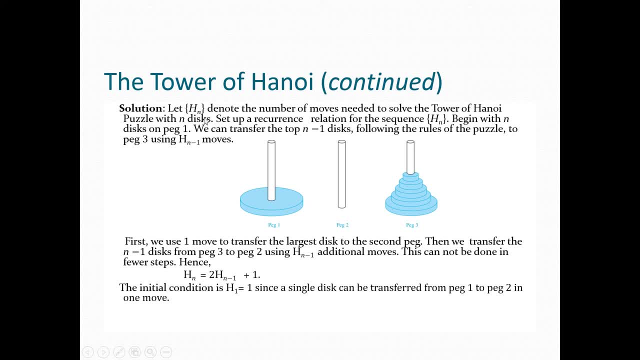 disks, because we have assumed that h n moves are required to arrange n disks. So n minus 1 disks are arranged on peg 3.. So h n minus 1 moves were required to do this. Now we use one move to transfer this. 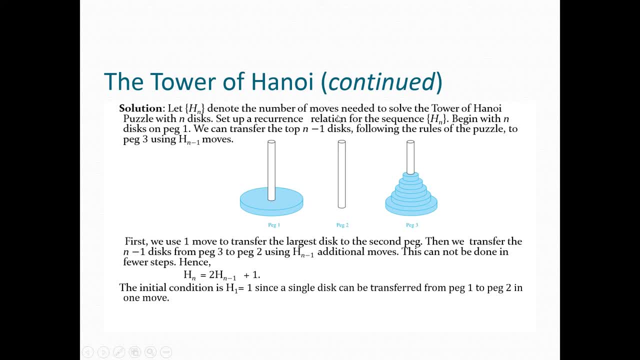 This peg onto peg 2, sorry, transfer this disk onto peg 2.. So one move is required to move this. So, and now we are left with n minus 1 disks to rearrange. So how many moves are required? 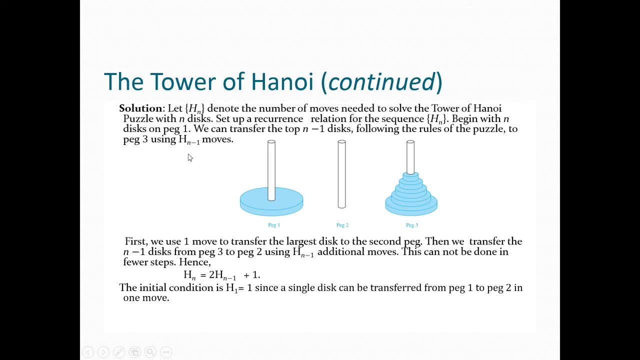 to arrange n minus 1 disks, h n minus 1.. So we have already used h? n minus 1 moves, 1 n minus 1 moves. So we have already used h? n minus 1 moves. So we have already used. 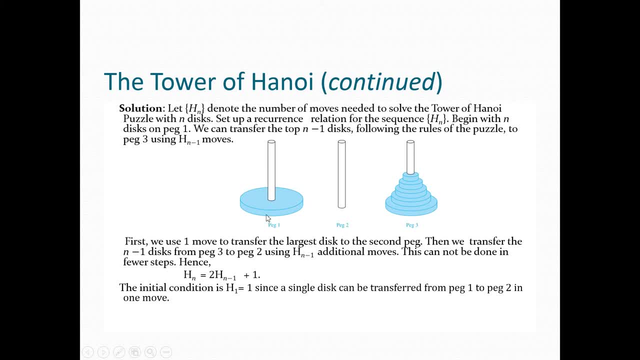 one move is used to transfer this disk to this peg, And then we have to transfer all these n��, these n minus 1 disks to this peg in the similar fashion. So how many moves are there in total? Two times hn minus 1 plus 1.. S o hn as n number of n moves needed to solve the Tower of Hanoi estasle. 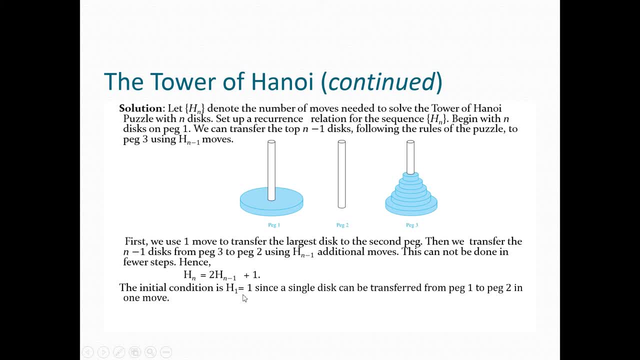 with n belongs to n minus 1 and this is focusing on n minus 1. so i is telling h n. so the n moves disks is equal to 2 times Hn minus 1 plus 1 and the initial condition is H1 is equal to 1.. 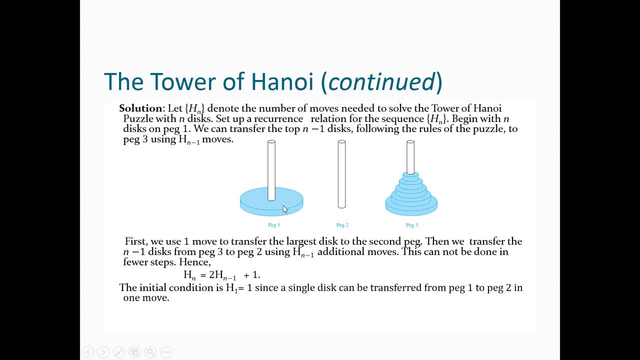 That is, if we have one disk. so we need only one move to transfer this disk to the pack 2, right? So H1 is equal to 1, because only one previous term is used in this recrystallation. So 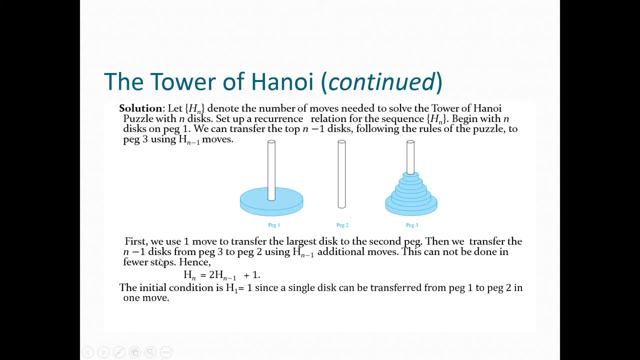 in order to proceed further, we just need one initial condition, okay, So, which is: H1 is equal to 1.. Now see if we have two disks, what is going to happen, For n is equal to 2, H2, that is number. 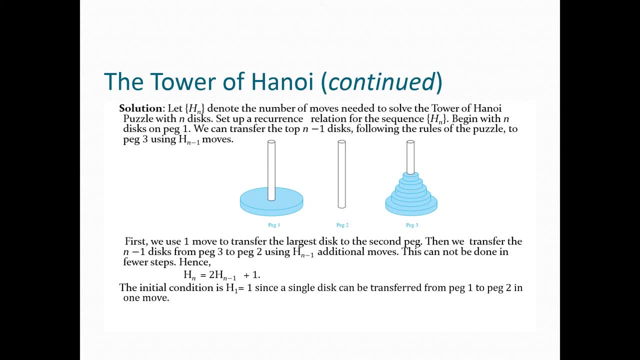 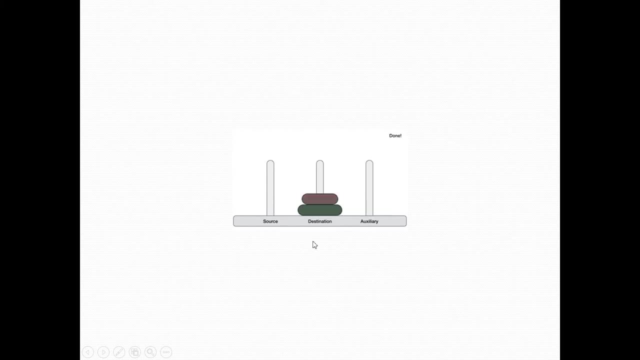 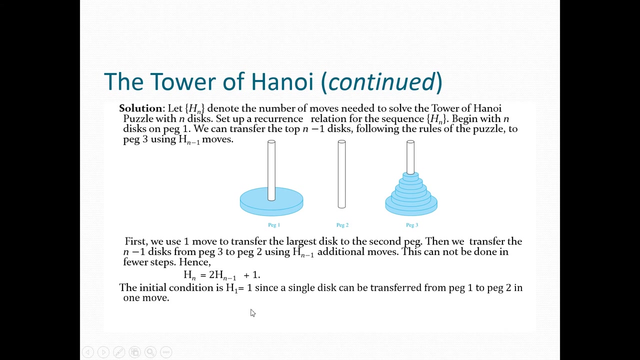 of arranging two disks in the required arrangement is equal to 2 multiplied by H1 plus 1, that is 3.. Okay, Okay, Okay. So I just showed you that only three steps are required to arrange two disks. See Yes, And H2 is now 3, okay, Now we know that H2 is 3.. So H3.. H3 is equal to 2 multiplied by 3. 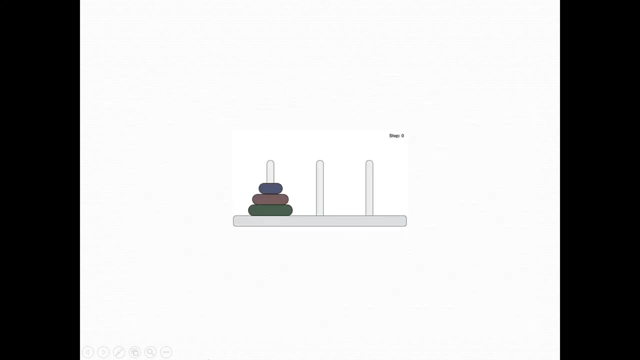 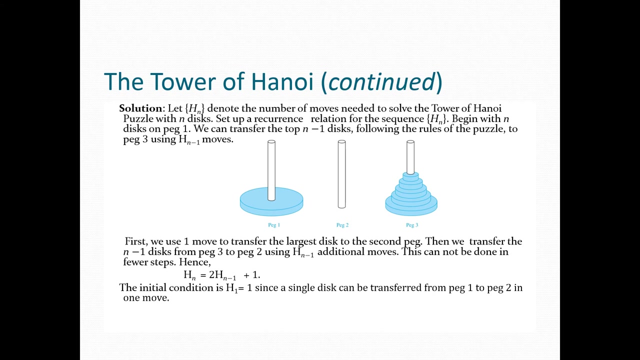 which is 6,. 6 plus 1, that is 7, okay. So I showed you before that we need 7 steps to arrange the disks. if we have three disks, okay, And similarly you can see for four disks, and this is the formula. 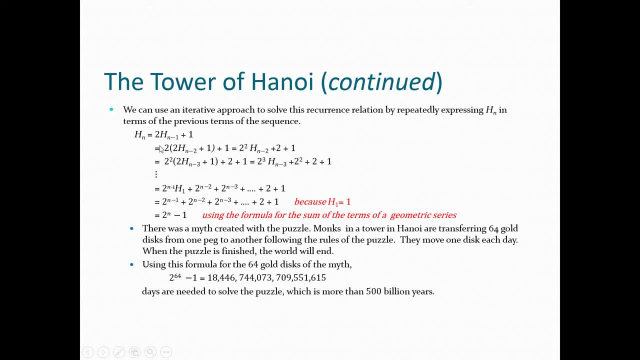 for n disks. okay, Now Hn. so we have this recrystallation: Hn is equal to 2Hn minus 1 plus 1.. Now if we want to get rid of this H and we just want to have a formula which depends upon: 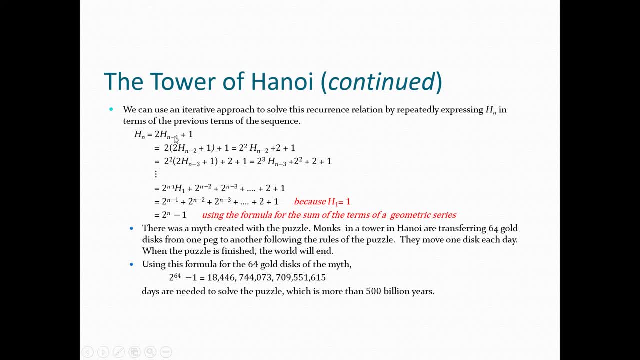 the number of disks, that is n. okay, So for this, what we are going to do, we are going to replace this Hn minus 1 by 2Hn minus 2 plus 1, because Hn is equal to 2Hn minus. 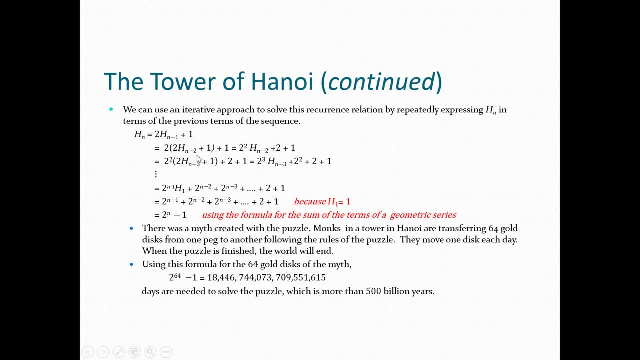 1 plus 1.. So Hn minus 1 is equal to 2Hn minus 2 plus 1.. Just replace n by n minus 1 in this formula, right? So we have this Now. this is equal to just simplify it, and we have this So. 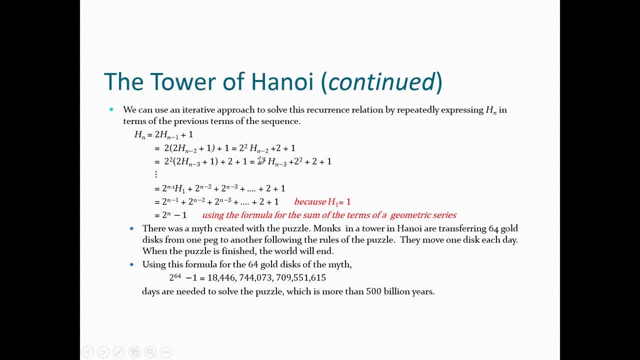 we have 2 square Hn minus 2 plus 2 plus 1, okay, Now replace Hn minus 2 using this formula by 2Hn minus 3 plus 1, and rest is as it is. So 2 square, just Hn minus 1, 2 is replaced by this plus 2 plus. 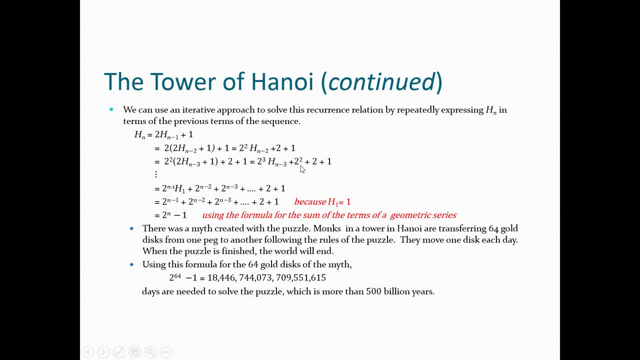 1 as it is. So we have 2 cube Hn minus 3 plus 2 square plus 2 plus 1, okay, And continuing this way, we have 2 to the power n minus 1.. Now you can see that 2 square and this subscript is n minus 2, 2 cube and this subscript is n minus 3.. 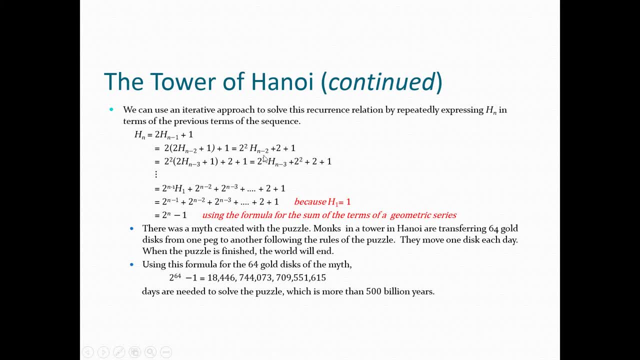 So it means, if you add this power and this subscript, we have n. okay, Add this power and this subscript, we have n right. So with H1, we must have 2 power, n minus 1, right 2 power. 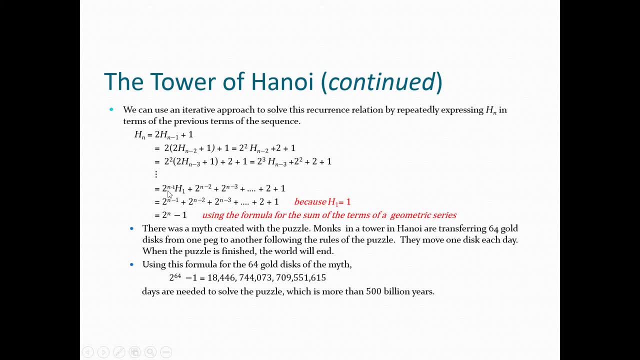 n minus 1, because by adding n minus 1 and 1, we have n? 2n minus 1, H1 plus 2Hn minus 1 plus 2Hn minus 2, and you can also observe that the powers of 2 are decreasing by 1 in every term. 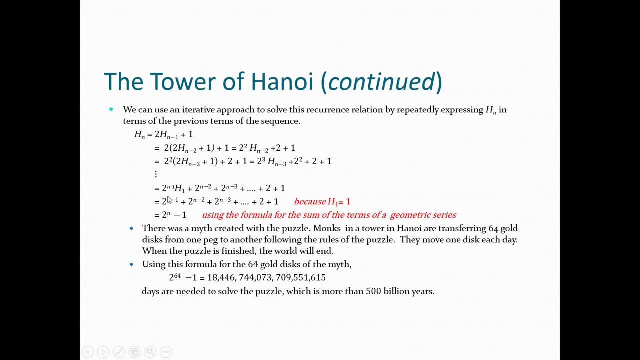 after the first term: right. So 2n minus 1, H1 plus 2n minus 2.. So powers of 2 are decreasing by 1 plus 2n minus 3, and so on. after 2 plus 1, okay, Now H1 is 1.. 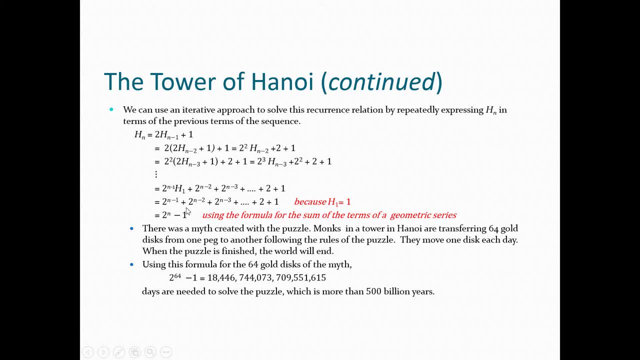 Just discovered that H1 is 1. H1 is the number of shifting 1 disk to the pack 2.. So it can be done in one move. So H1 is 1. 2n minus 1 plus 2n minus 2. So we have this sum of. 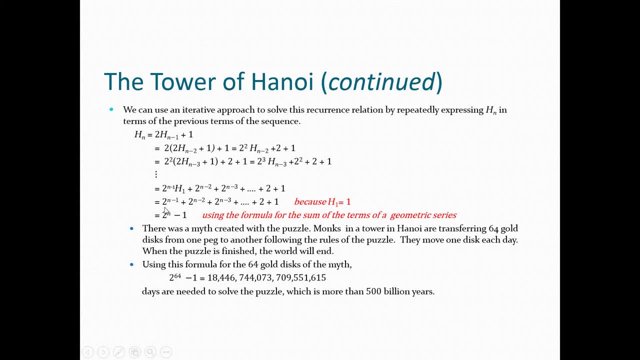 geometric sequence: wow, right. So this is first n terms. first n terms: yes, 2 to the power 0 and we add up till 2 to the power n minus 1.. So we have first n terms sum of the first n terms of the geometric series. So the formula: 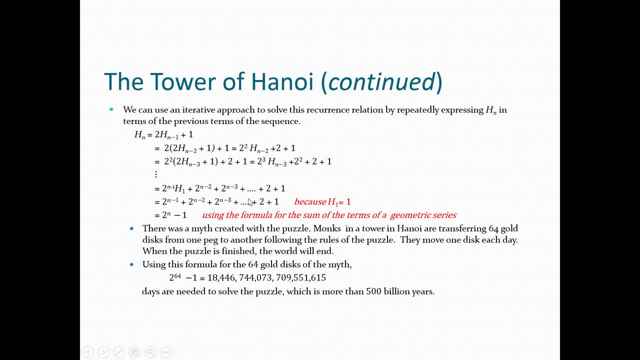 is with the common ratio 2, or rather 1 over 2, right So 1 over 2.. If the first term is 2 to the power n minus 1, we have 1 over 2, and if the first term is 1, we have 2, and if the first term is 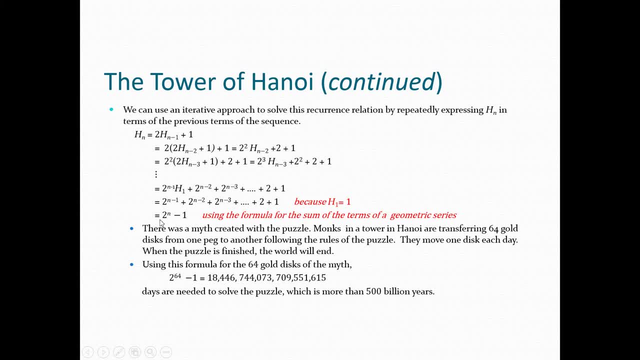 1, you can use the formula to have: the value of this sum is equal to 2n minus 1, and you know the formula. just apply it and you will get this sum 2n minus 1.. So Hn is equal to 2n minus 1. in other, 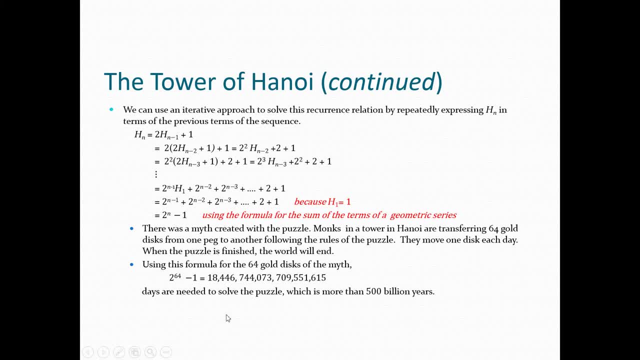 words. okay, So there are few interesting observations. There was a myth created with the puzzle mocks in a tower in Hanoi, So they were transferring 64 gold discs from one pack to another following the rules of the puzzle, and they move one disc each day and when the puzzle is finished, the world will end, okay. 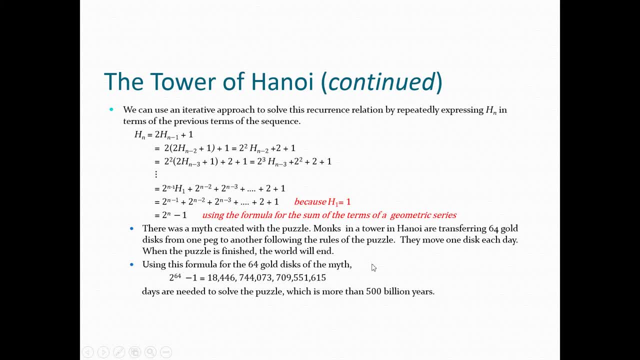 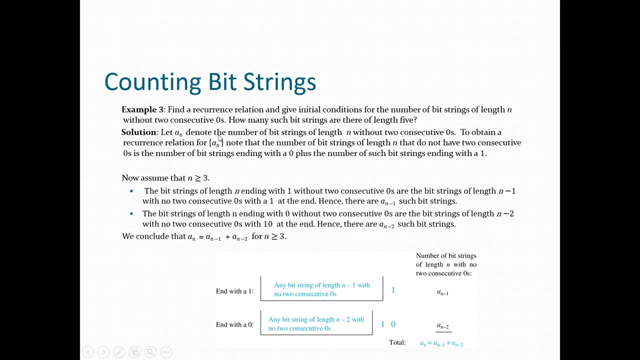 So, using this formula, these much days are required to end the world, and this is actually 500 billion years. So kyaamath is too far according to this myth, okay, Okay, let's have an example of establishing a recurrence relation. First example, which is example number: 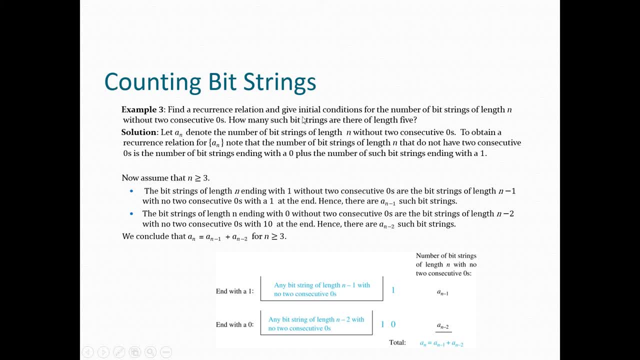 3 of your book. find a recurrence relation and give initial condition for the number of bit strings of length n without two consecutive zeros, right, How many such bit strings are there of length 5?? So find a recurrence relation. let me read it again: find a recurrence relation and. 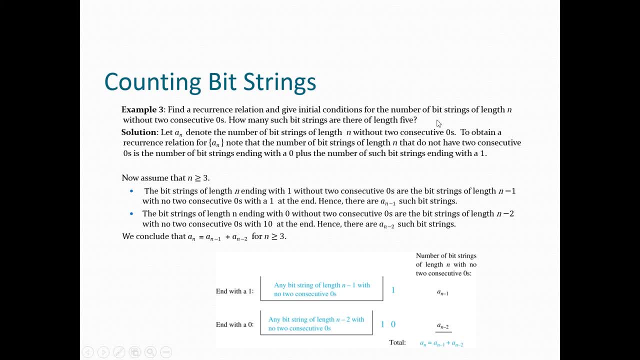 give initial condition right For the number of bit strings of length n. so we have to form the number of bit strings of length n now with the condition without two consecutive zeros- the string should not contain consecutive zeros- right? So how many such bit strings? 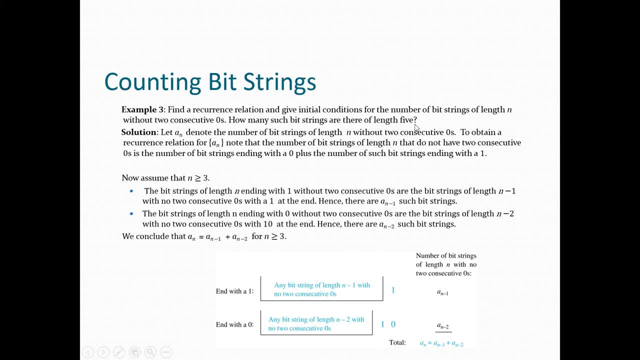 are there of length 5?. So initially we have to develop a recurrence relation right For and for this, and then we have to find the number of bit strings of length 5, with the condition that there are no consecutive zeros, two consecutive zeros. So let a n denote the. 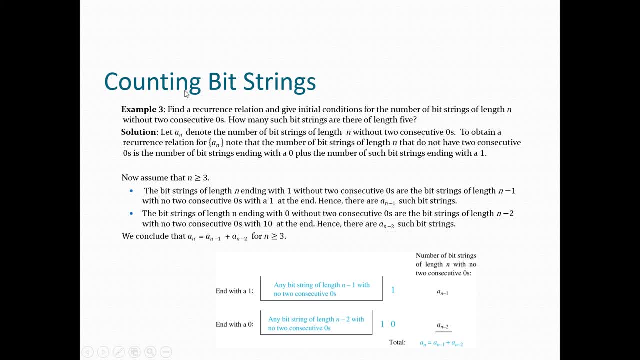 number of bit strings. Since we have to find the number of bit strings, so we denote a- n, the number of bit strings of length n, without two consecutive zeros. So obtain a recurrence relation for a? n, the sequence a- n. Note that the number of bit strings of length n that do not have 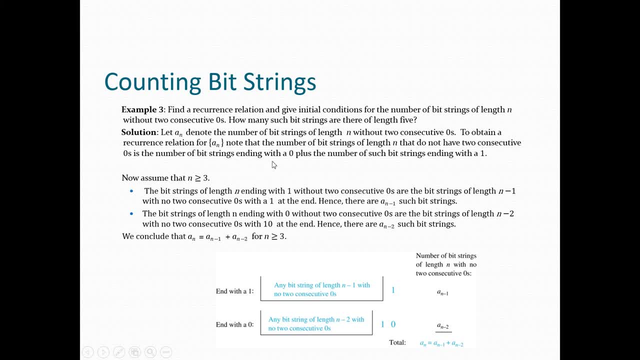 two consecutive zeros is the number of bit strings ending with a 0, okay, plus the number of bit strings ending with a 1.. Of course, if you have bit string, it can end with a 0 or it may end with a 1.. 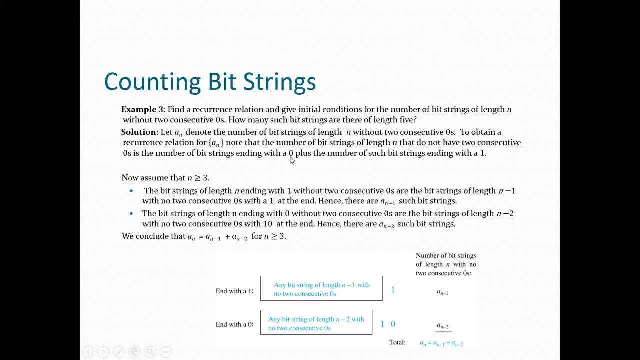 But if it ends with a 0, it cannot be ended with double 0. So it will end up with 1: 0, okay. So if it ends with 1, then this is okay. we are left with n minus 1 spaces, and if we 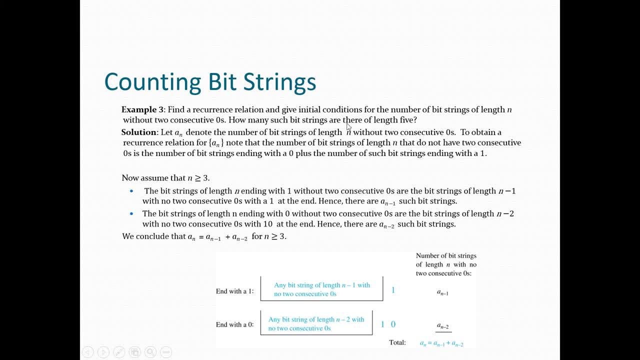 end up with a 0, then, since two consecutive zeros are not allowed, so we will end up with 1: 0,. okay, In this case we will have n minus 2, length: n minus 2 bit strings, okay. And in this case, 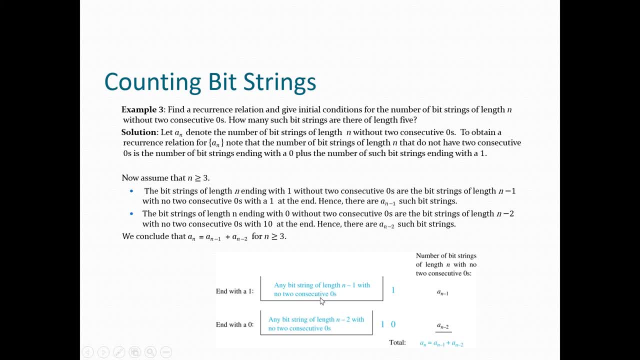 we have to find the number of n minus bit strings of length n minus 1, with no consecutive zeros. okay, two consecutive zeros. So what to do? The bit strings of length n ending with 1 without two consecutive zeros are the bit strings of length n minus 1.. So what to do? 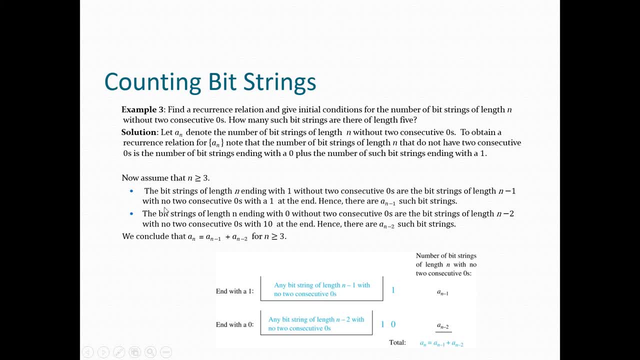 So what to do? The bit strings of length n ending with 1 without two consecutive zeros are the bit strings of length n minus 1, as I just said, with no two consecutive zeros, with a 1 at the end. Hence, there are a n minus 1 such bit strings, because we assumed that a n be the number of. 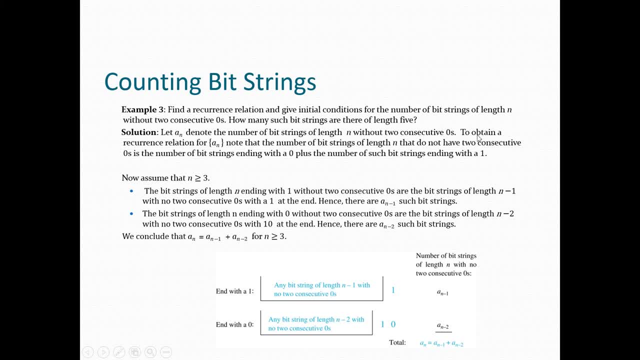 bit strings of length n without two consecutive zeros. So if we have to form the bit strings such bit strings of length a n minus 1, then the number of bit strings must be a n minus 1.. Okay Now, the bit strings of length n ending with 0 without two consecutive zeros are the 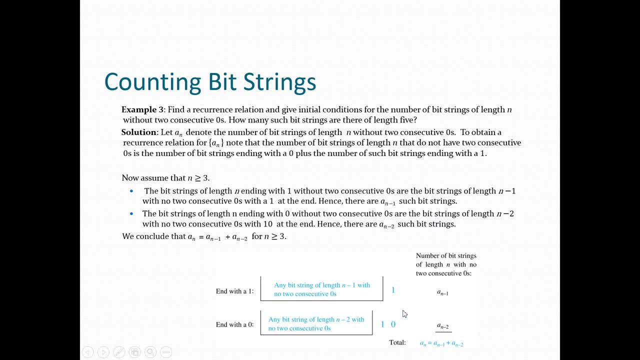 bit strings of length n minus 2, because they must end like 1, 0. So we are left with n minus 2, actually spaces. So these are the length of length. So the remaining length of the bit string is n minus 2.. So the 2 bit strings, let me. 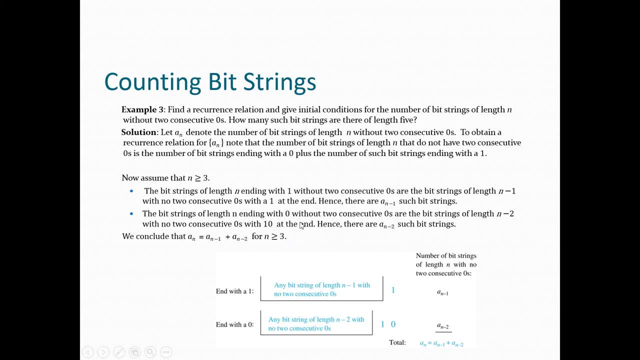 read, I am lost. The bit strings of length n ending with 0, without two consecutive zeros, are the bit strings of length n minus 2, with no two consecutive zeros, with 10 at the end, of course, 1, 0 at the end. Hence there are a n minus 2 such bit strings. the same logic. 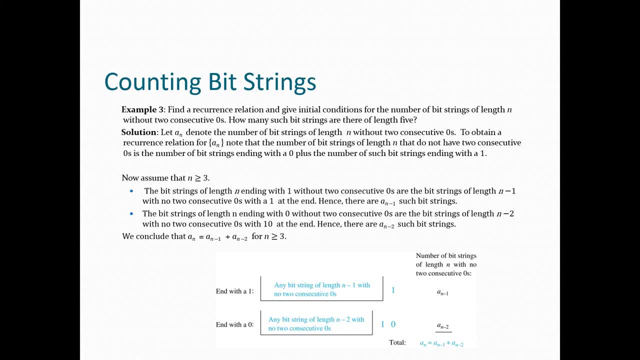 because the number of bit strings of length n is a n. So a number of bit strings of length n minus 2 is a n minus 2.. Now the total number of the bit strings of length n, without two consecutive zeros, is the sum of these two numbers. right, because there is, there are. 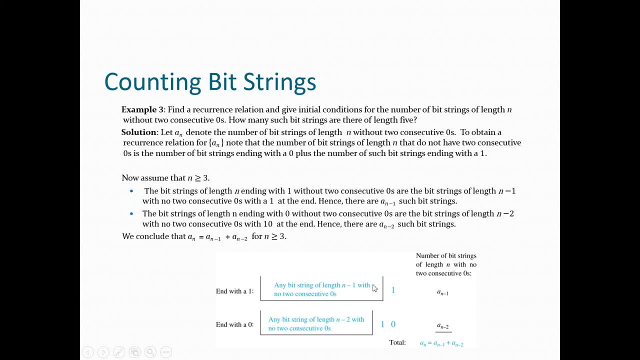 only two possibilities to have such bit strings. So the number of bit strings with 1 at the end is a n minus 1.. The number of bit strings with 1, 0 at the end is a n minus 2.. So the 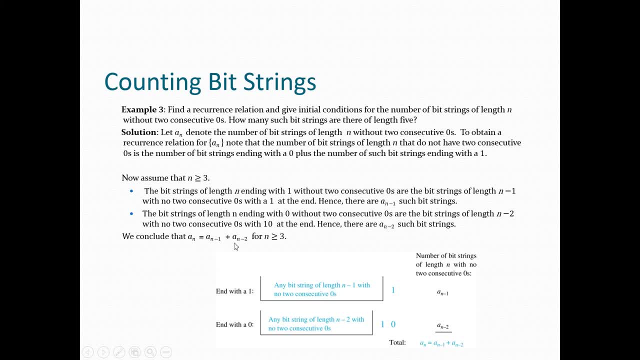 total number is the sum of these two numbers, that is, a n minus 1 plus a n minus 2.. So a n is equal to a n minus 1, a n minus 2 for n greater or equal to 3.. Now, in order to 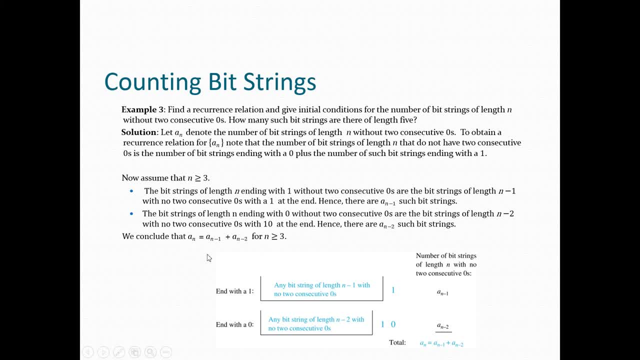 initialize the process and in order to find the a n for the particular values of n, we need to have a 1 and a 2, because previous two terms are used to find the n minus 1.. So the number of bit strings with 1, 0 at the end is a n minus 2.. So the total number 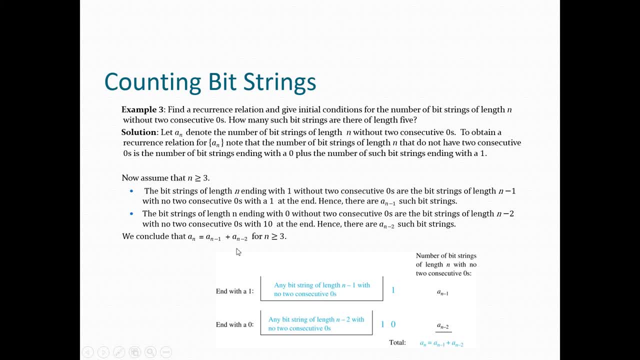 is the sum of these two numbers, that is, a n minus 1 plus a n minus 2.. So a n is equal. terms are used to find the next term. So what is the value of a1? a1, that is, if we. 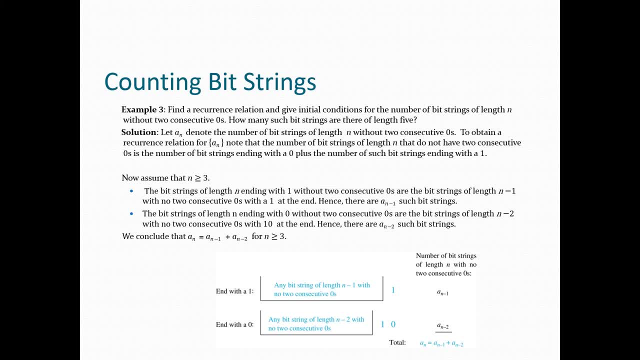 have a bit string of length 1 and we cannot have consecutive zeros. So a1 is 1.. And what about a2?? a1 and a2 are required to start with this reconciliation to find the values of a1.. So a2, that is a bit string of length 2.. Bit string of length 2. the possibilities are: 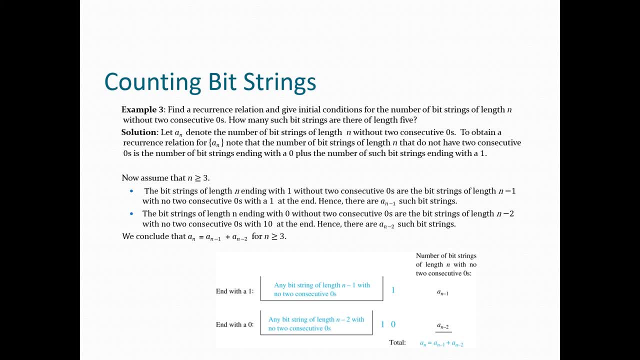 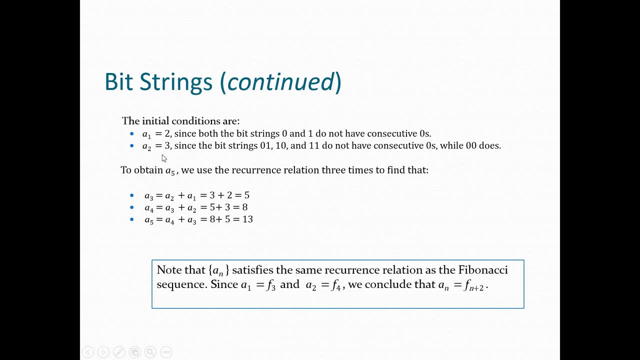 1: 0,, 0, 1,, 1: 1 and 0: 0. But 0: 0 is not allowed. So we have three possibilities. So a1 is 2 and a2 is 3.. Oh yes, a1 is 2.. What I said, a1 is 1?? No, a1 is 2. Because 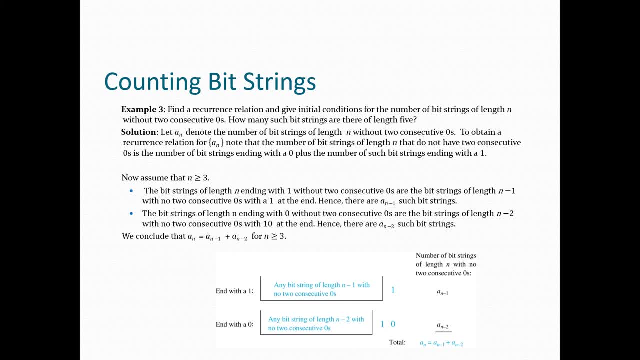 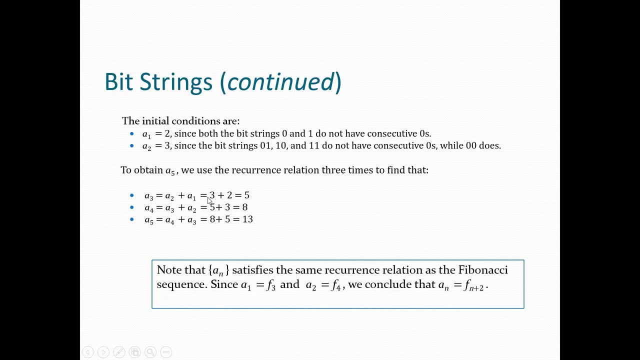 a bit string of length 1 can be either 0 or 1. So a1 is 2 and a2 is 3.. So next part of the question was: how many such bit strings are there of length 5? So how many such bit strings? So? 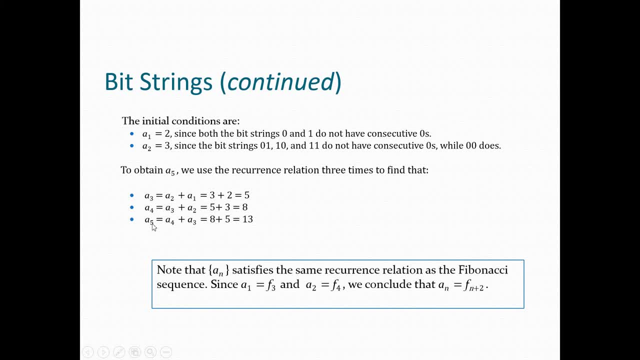 we have to find all the number before finding a5. So we have to find a3, we have to find a4, and a3 are used in order to find a5. So first we will find a3, then a4, then a5, and a5 is 13. 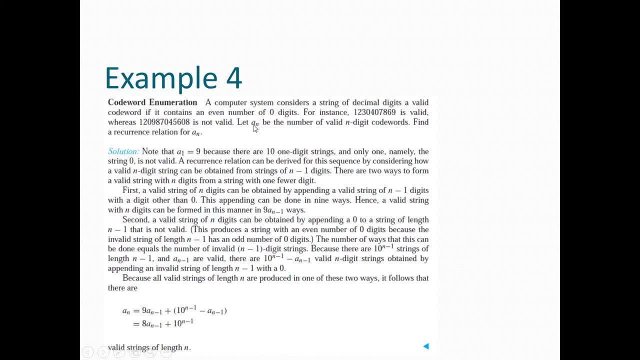 using the formula. Next example, number 4.. A computer system considers a string of decimal digits a valid code word if it contains an even number of zeros, For instance 1,, 2,, 3,, 0,, 4, 0,. 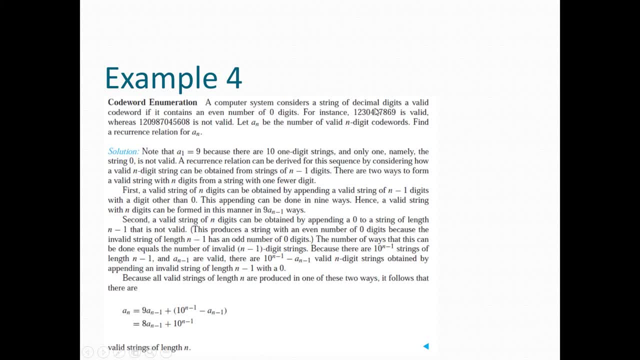 7,, 8,, 6, 9.. Now contains two zeros. that is even number of zeros. This is valid, Whereas this code word, which contains 1,, 2, 3 zeros, is not valid. Let a? n be the number of valid and dated code words. Find. 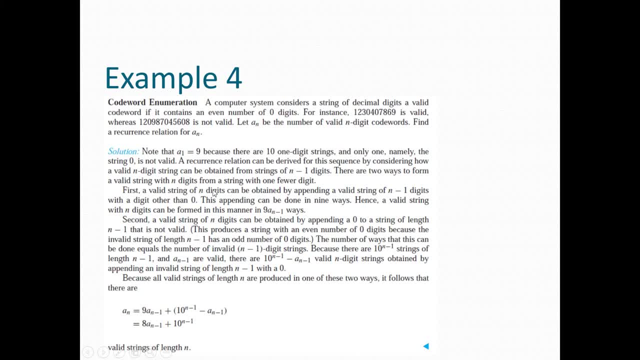 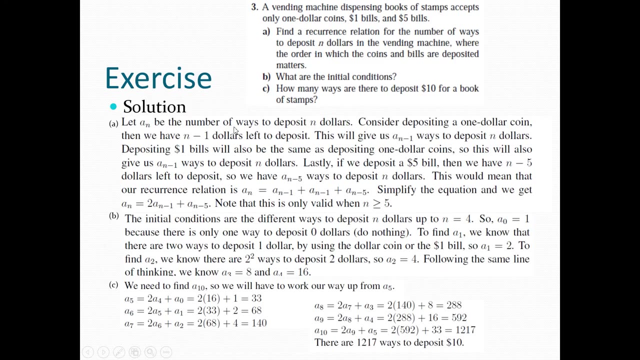 the reference relation for n And this is an example. 4, which is solved in your book. You can read it and you can easily find this formula. If that is an issue, you can let me know and we will discuss it on Monday. So let us solve few questions from exercise. There is question. 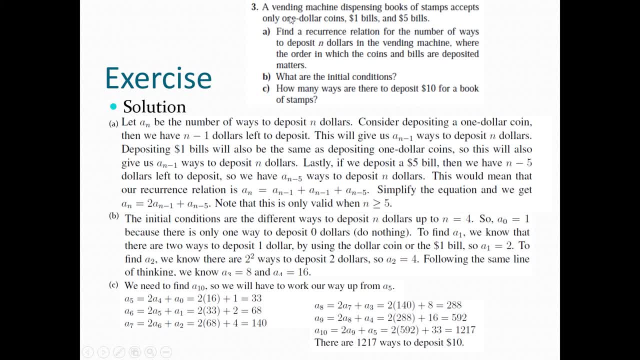 number 3 from the exercise A: vending machine dispensing books of stamps except only one dollar coins, one dollar bill and a five dollar bills. Find a reference relation for the number of ways to deposit n dollars in the vending machine. The order in which the coins and bills are deposited matters. Part b. What are the initial? 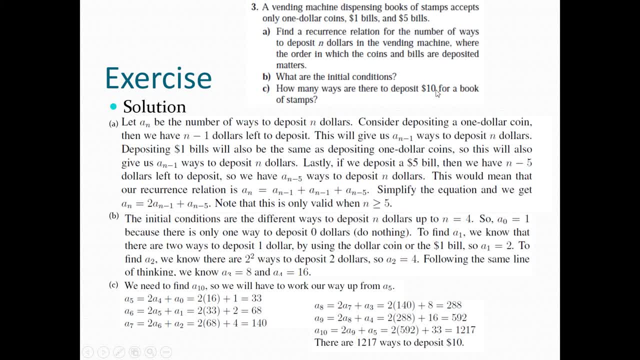 conditions. Part c: How many ways are there to deposit 10 dollars for a book of stamps? Okay, So let us start with an assumption that a? n be the number of ways to deposit n dollars. Okay, Now consider depositing one dollar coin. Okay, 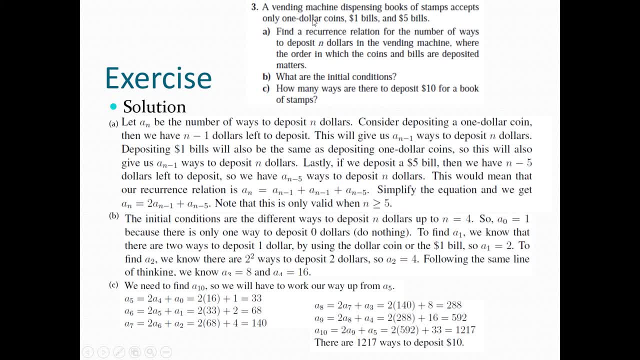 So if we start with one dollar coin, then see how many options are there. So how many ways are there. if we start with one dollar coin, Okay, Consider depositing one dollar coin. then we have n minus dollars left to deposit. Okay, And n minus 1 dollars can be. 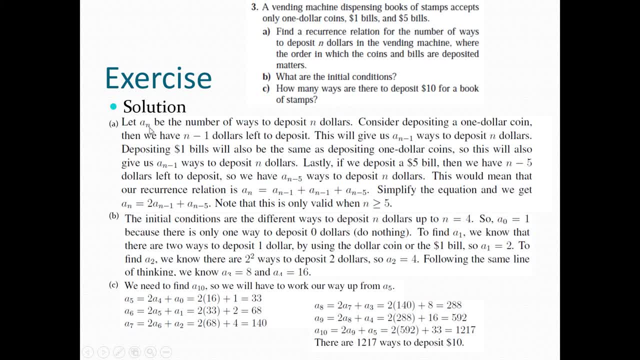 deposited in a n minus 1 ways. Okay, So these n ways can be deposited, can be done in a way, or these n dollars can be deposited into 1, multiplied by a n minus 1 ways. right, so this will give us a n minus 1 ways to deposit n dollars. i i hope it makes sense now. second way: 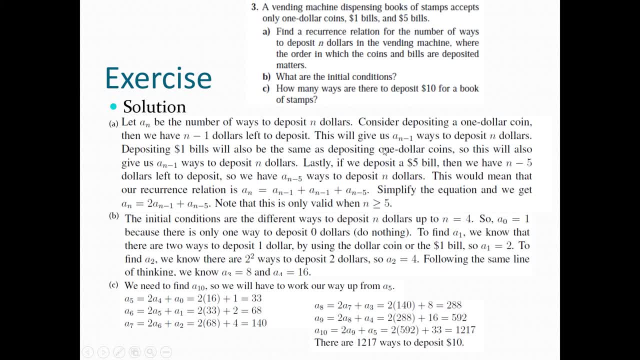 in this way. in this way, we started with one dollar point. now, if we started start with one dollar bill, then what happens? so depositing one dollar bills will also be the same as depositing one dollar coin. so this will also give us a n minus 1 ways. okay, if we deposit one dollar bill. 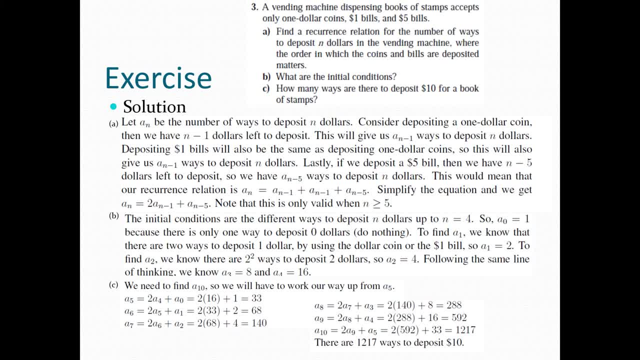 then we are left with again n minus 1 dollars, and it can be done in a n minus 1 ways. so total number of ways are 1 multiplied by a n minus 1. so a n is. in this way n dollars can be deposited in. 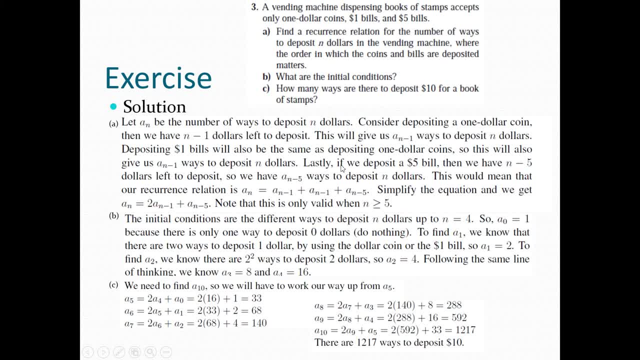 a n minus 1 ways. so, lastly, if we deposit a five dollar bill, then we have n minus five dollars left to deposit, right, so we have a n minus 1 ways to deposit n dollars, because a n is the number of ways to deposit n. 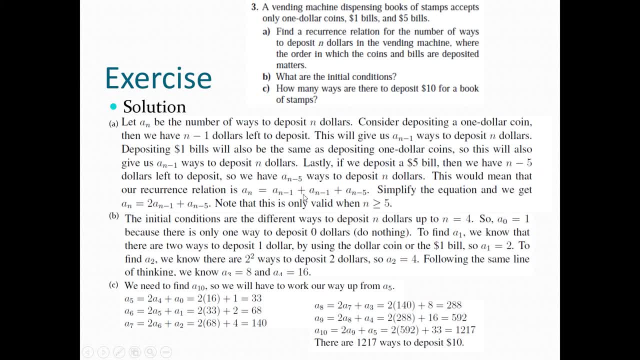 dollars. now we have n minus 1, five dollars to deposit. so there are a n minus 5 ways to deposit n dollars. so this would mean that our recurrence relation is a n. now total number of ways is equal to a n minus 1 plus a n minus 1 plus a n minus one. so all the options are added, okay. 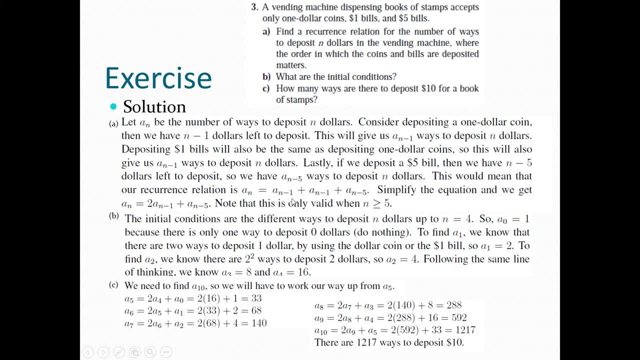 the number of ways for all the options is added to have the total number of ways to deposit ten dollars. now simplify the equation. we have two times a n minus one plus a n minus five. now see a n minus five is used. so we must know to initialize the procedure. a 1, a 2. 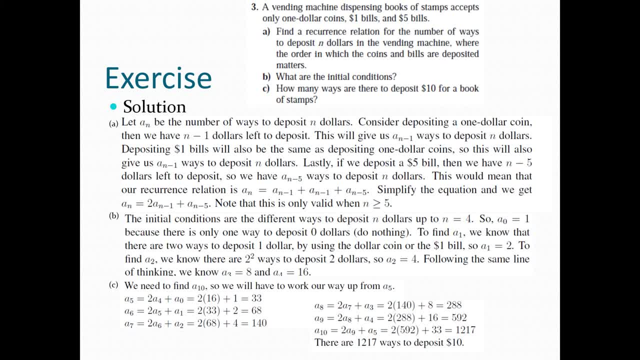 a3, a4 and a naught as well. if we have i mean nothing to deposit, then what happens? so the initial conditions are. next part is: what are the initial conditions? the initial conditions are different ways to deposit. 10 dollars up to n is equal to 4, so a naught is equal to 1, because when we 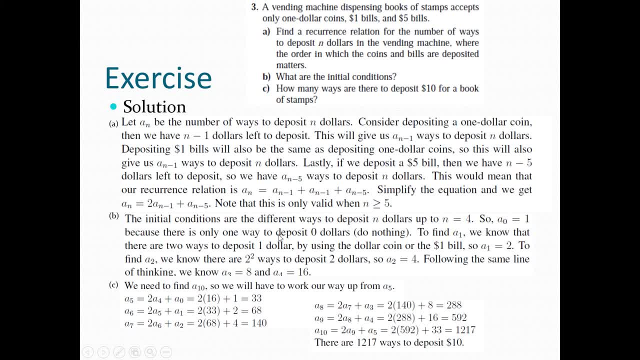 have nothing to deposit, then there is only one way that we are not going to do anything. so to find a1, we know that there are two ways to deposit one dollar: by using one dollar coin or, uh, the one dollar bill. so this or makes it this the addition problem. so addition counting: 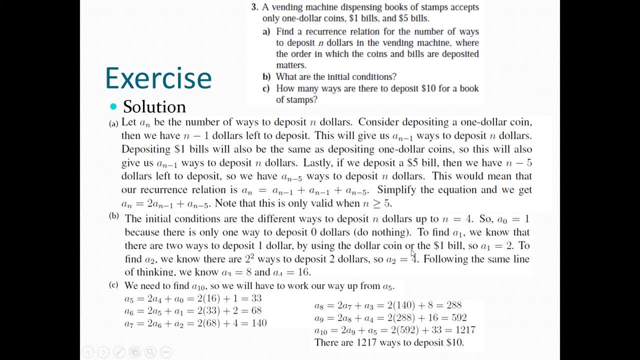 you learned this addition law in chapter 6, yes, so this, or actually tells us to add both the ways. so we have: a1 is equal to 2, so to find a2, we know there were two square ways to deposit two dollars or so a2 is equal to 4. okay, so, following the same lines of thinking we have. 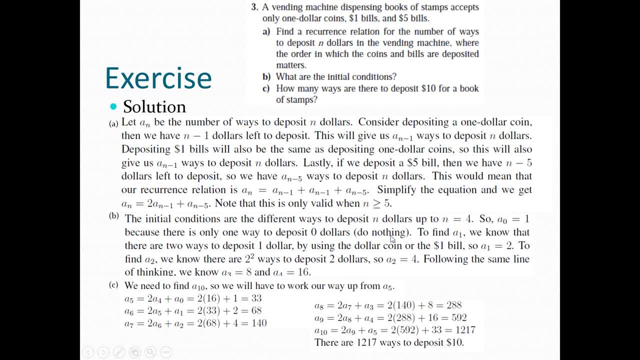 a3 is equal to 8 and a4 is equal to 16. so these are the initial conditions. now we need to find a10. and in order to find a10, uh, we need a9, we need a5, so we have to find all these before finding a10. so, uh, using this formula, uh, we'll just plug in the values and: 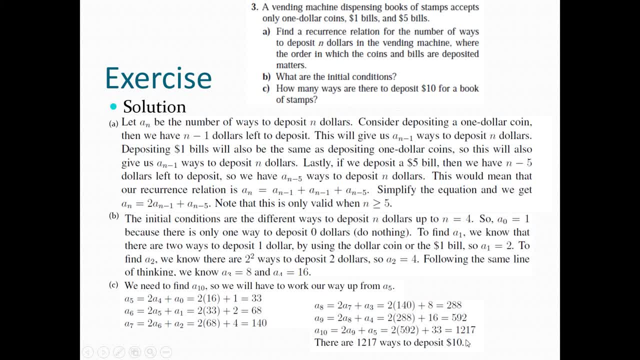 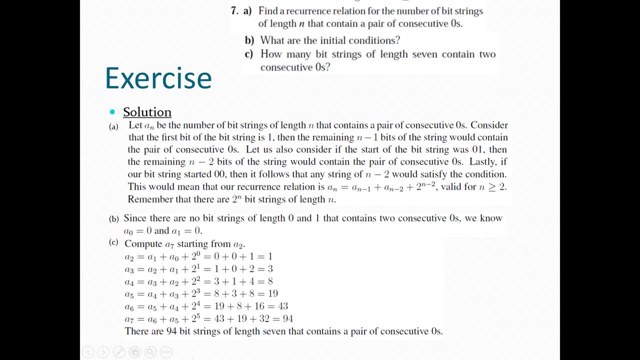 ultimately we have, a10 is equal to 1 to 1: 7. okay, so there are 1 to 1: 7 ways to deposit 10 dollars. now question number seven. from the question number seven, we need to find a10. and in order to find a10, 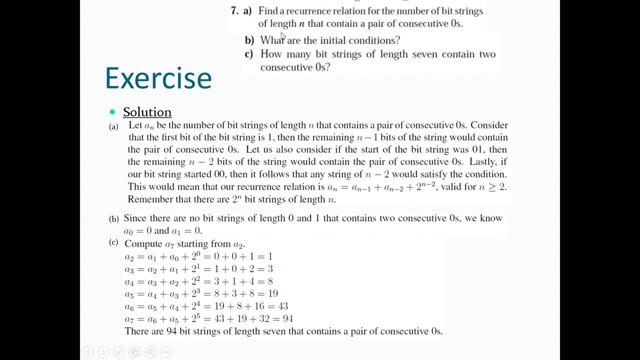 we will divide the parentheses between these two 코를 and Sütлатomi에도 파이 같은데, uh, to use between CaN x faN, y x bar versus N 2 x bar. Okay, let's solve for the next couple of equations. 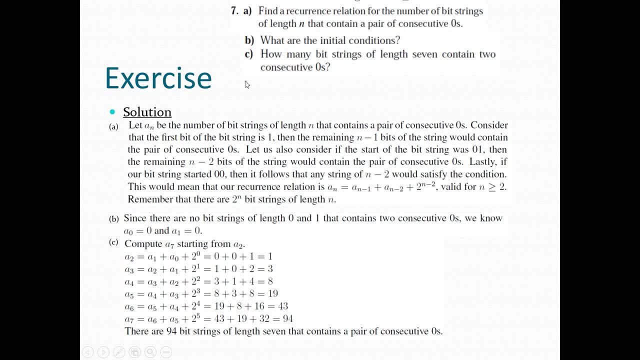 zeros, and part b, we have to find the initial conditions and in part c we have to evaluate what. how many bit strings? okay, uh, we have to evaluate a7. if a- n be the number of strings of length n containing pair of consecutive zeros, okay, let's start the solution. let a- n be the 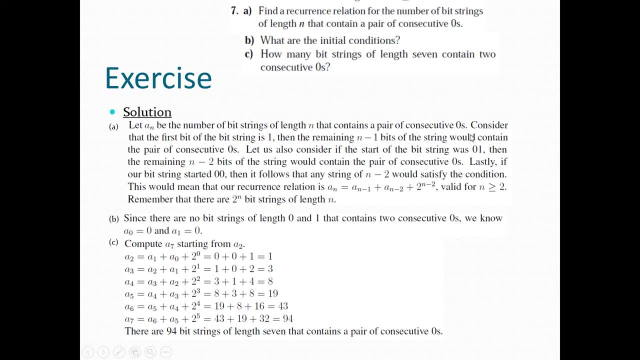 number of bit strings of length n that contains a pair of consecutive zeros. consider that the first bit of the bit string is one. okay, then the remaining n minus one bit string would contain the pair of consecutive zeros. right? let's also consider if the start of the bit string 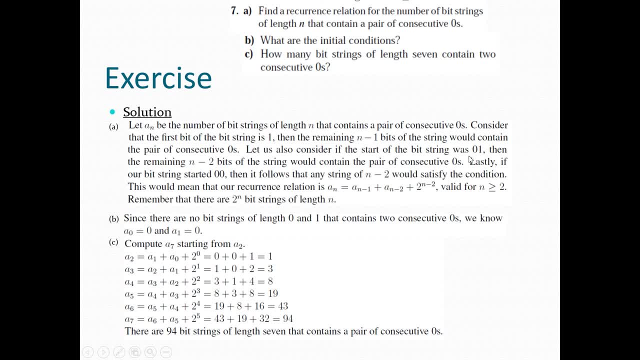 was zero one. okay, a bit string can be started from one or zero. if it starts from one, then the remaining n minus one bits of the string, the string would contain a pair of consecutive zeros. or if it starts with zero, then there are two possibilities. either it starts with double zero, then there is nothing to actually show. 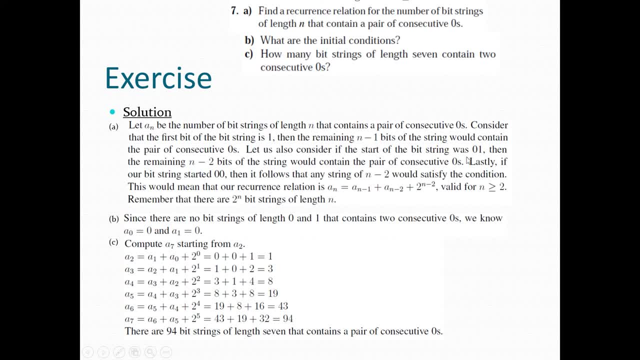 it contains a pair of zeros, and what if it starts with zero one? so let's also consider: if the, if it starts the, if the start of the bit string was zero one, then the remaining n minus two bit strings would contain the pair of consecutive zeros. and lastly, if our bit string started zero, 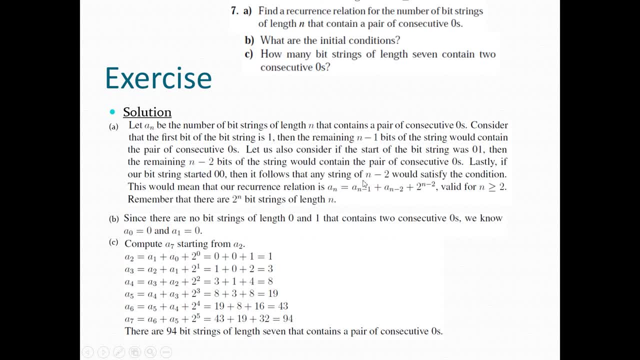 zero. so third option: then it follows that any string of n minus two would satisfy the condition. okay, so it's already done. uh, it contains, uh, we don't need to look uh into the next uh bits. so, uh, a bit's number of bit strings would contain a pair of consecutive zeros. and lastly, if our bit string 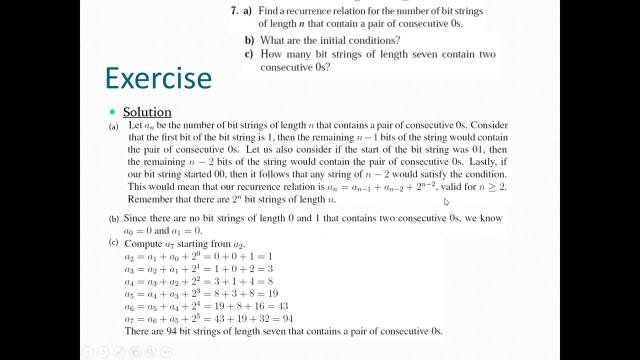 of length n minus two is two to the power n minus two. okay, so, uh, adding all these options, adding all these ways, we have a n is equal to a n minus one, plus a n minus two, plus two to the two power n minus two. and uh, here n is greater or equal to two because these previous two terms are used, so n is. 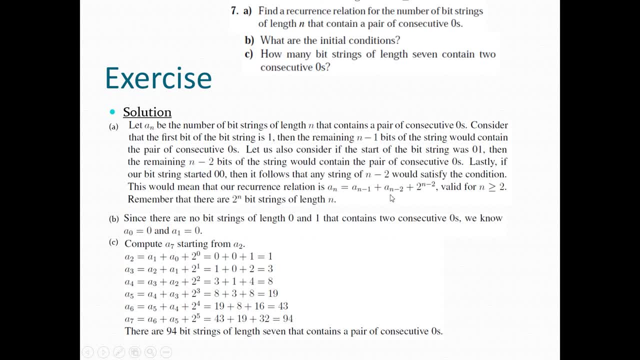 greater or equal to two. so we need to know the value of a naught and we need to know the value of a naught. that is a bit string of length. zero is zero. so a1 again, uh, a1, a bit string of length. one cannot contain a pair of zeros, of course. so a naught is zero, a1 is zero. 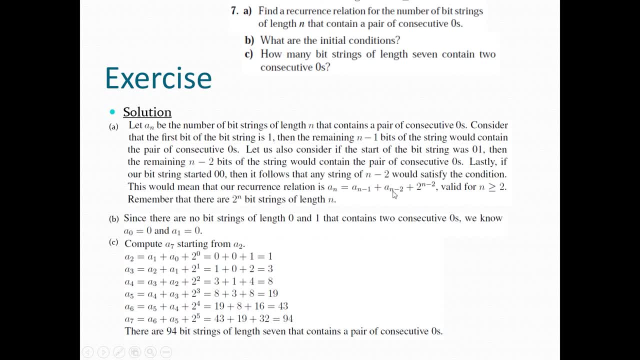 and then we can proceed with this relation in order to find any length, number of bit, strings of any length, right, and finally, we are required to find a7. so in order to find a7- we have- we must have the values of a6 and a5. so we have to find all the previous values and this ends up a7. 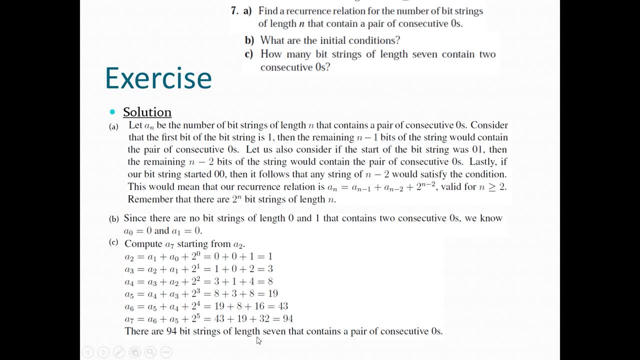 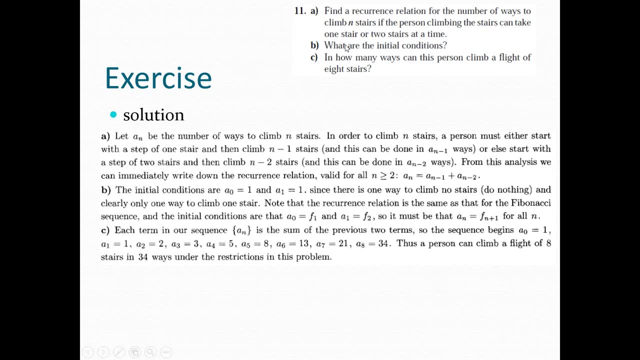 is equal to 94. so there are 94 bit strings of n7. you can do it yourself and to verify that. so question number 11: find a recurrence relation for the number of ways to climb n stairs if the person climbing the stairs can take one stair or two stairs at a time. so what are the initial conditions? 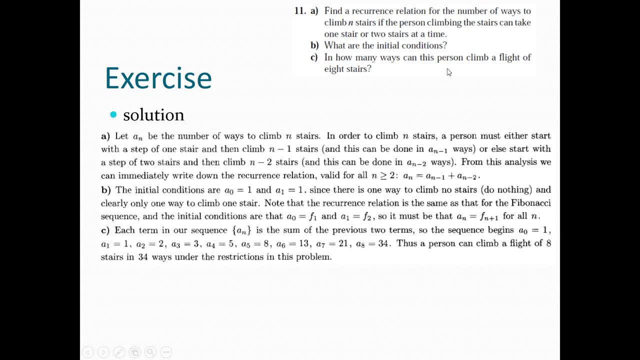 in how many ways can this person climb a flight of eight stairs? okay, so again, in the first part we have to establish the recurrance relation. in the second part we have to tell the initial conditions to initialize the procedure of uh finding a since國 tem 돌아가기. 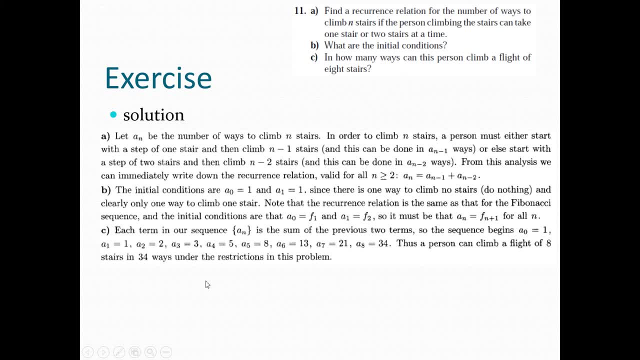 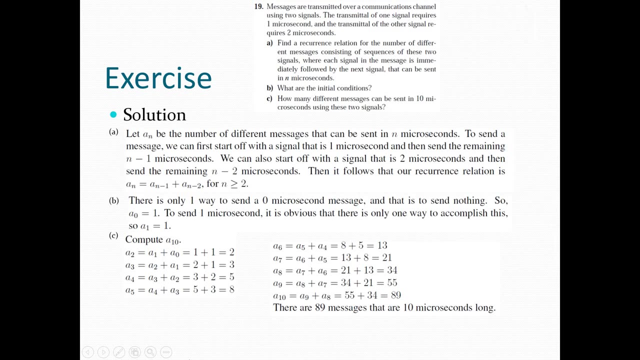 finding an and finally we have to find the value of a8. okay, and i'll share the solution in pdf form so you can do it yourself. solution is given here. i'm not going to explain it. next question, question number 19: messages are transmitted over a communication. 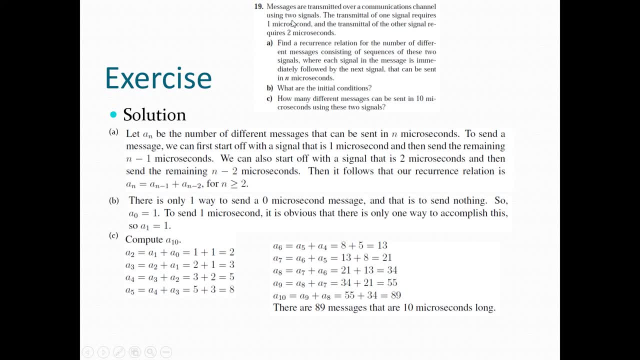 uh channel using two signals. okay, the transmittal of uh one signal requires one microsecond and the transmittal of the other signal requires two microseconds. so part a: find the reference relation of the number of different messages consisting of sequence of these two signals, where each signal 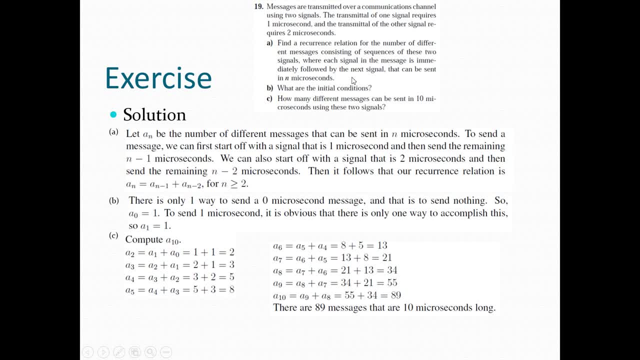 in the message is immediately followed by the next signal that can be sent in n microseconds. part b: what are the initial conditions? as always, we need initial conditions to initialize the process. and part c: how many different messages can be sent in 10 microseconds. that is, we have to find. 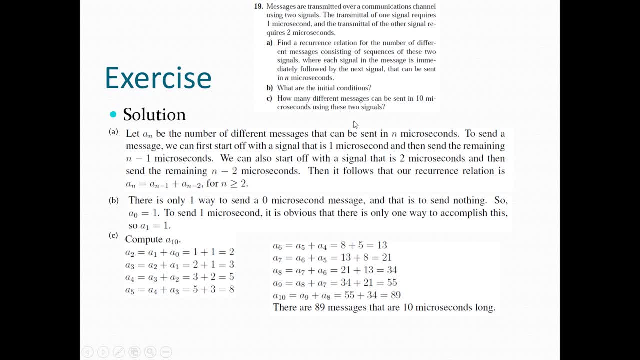 a n using these two signals. okay, so let's go through the solution. uh, let a n using this initial condition of the signal, and we will start with an unnumbered number of messages. as always, we assume the unknown thing: uh, the number of ways. unknown number of ways. 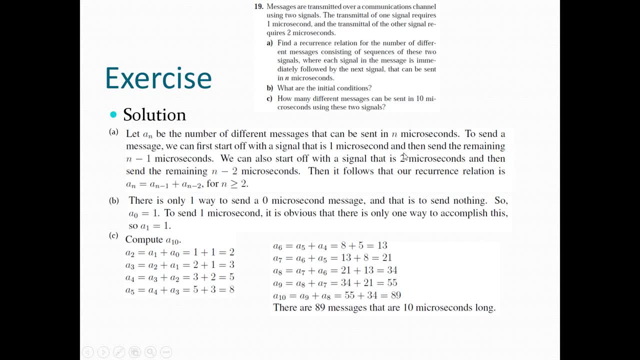 to be a n, so let a n be the number of different messages that can be sent in n microseconds. now, to send a message, we can first start off with a signal that is one microsecond and then send remaining and minus my microseconds- microseconds. then it follows that our recurrence relation is a. n is equal to a n minus 1 plus a n. 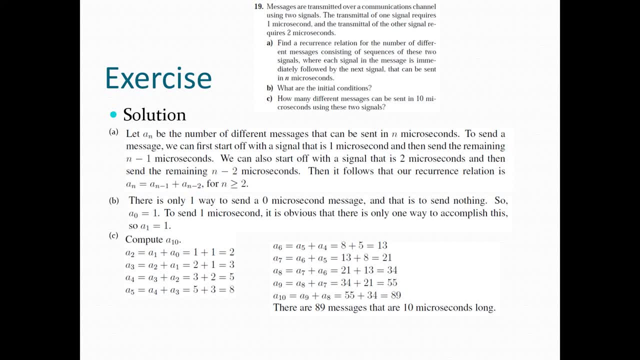 minus 2, right? so after doing so many examples, it makes sense now i think this needs no explanation, but still, if there is a confusion, you can ask me. uh, part b- initial conditions. so uh, two previous values are used, right? so we have, we need uh, two previous values, that is, two initial conditions. 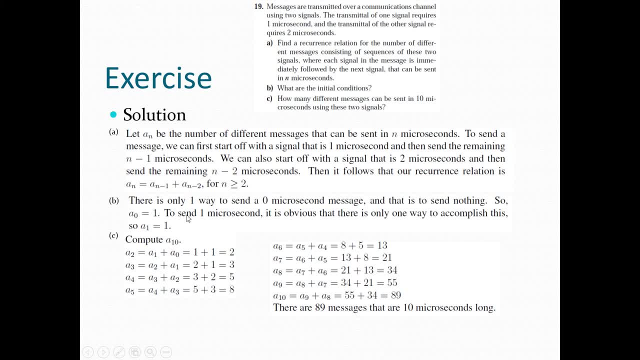 which is a naught and a 1. so there is only one way to send a zero microsecond message, that is, to send nothing. so a naught is one uh to send one microsecond. it is obvious that there is only one way to accomplish this. so a1 is equal to 1 and in order to find a 10, we have to find a 9.